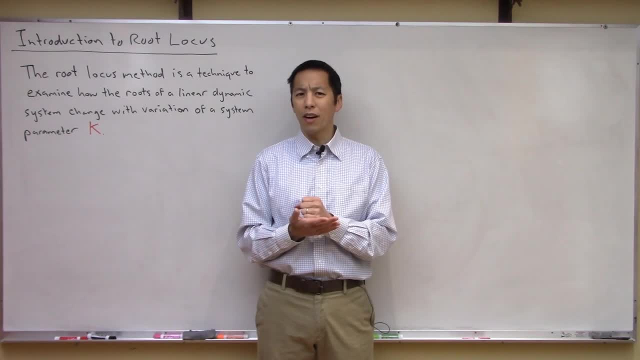 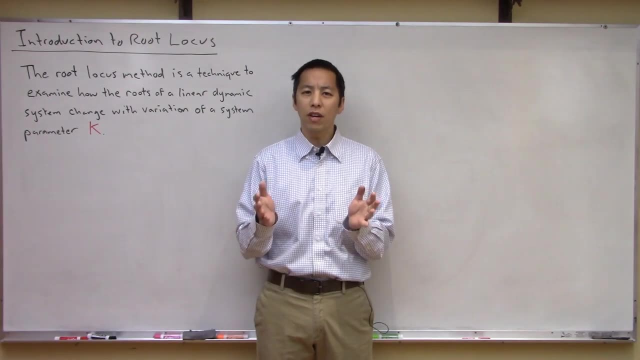 We're going to see that root locus. it really is set and based in one of the kind of classical engineering problems that you're always going to run into, Namely, if you're given a system you want to understand, how does that system change if I tweak some kind of parameter? right, 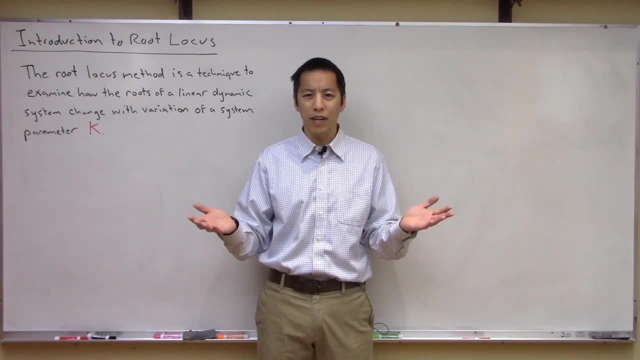 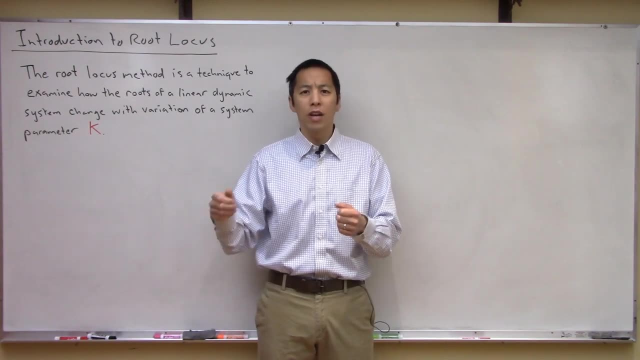 That's the classical engineer's dilemma, right? It's basically glorified Guess and check at some level where, if you get a system, you're just going to tweak it, tinker with it, change some small parameter and see how does that affect the overall behavior of the system. 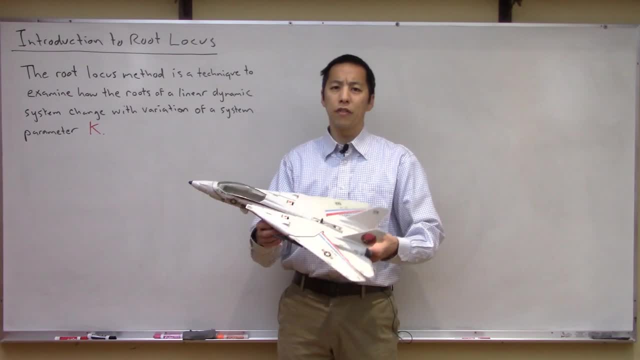 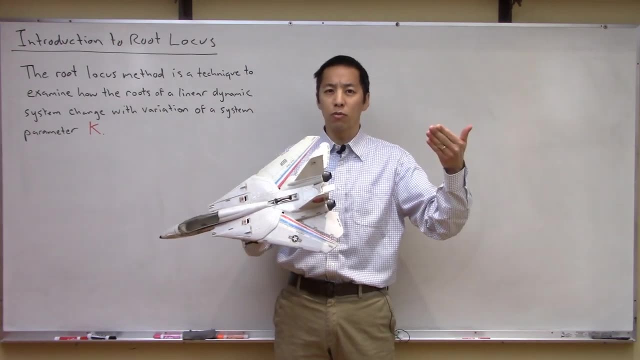 So, for example, I've got some props. Let's say, you've got an aircraft, right, You've got some aircraft configuration like this F-14. And now you want to ask: how does something about this system change if I change some other parameter? 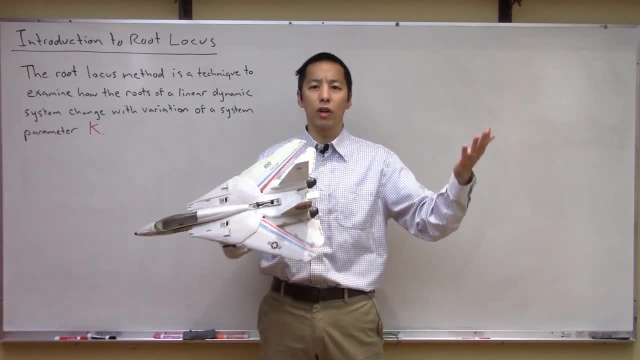 So, for example, how about let's look at the aircraft like endurance. How long can the aircraft stay? How long can the aircraft stay in the air? Well, in this configuration, it can probably stay up in the air for a certain amount of time. 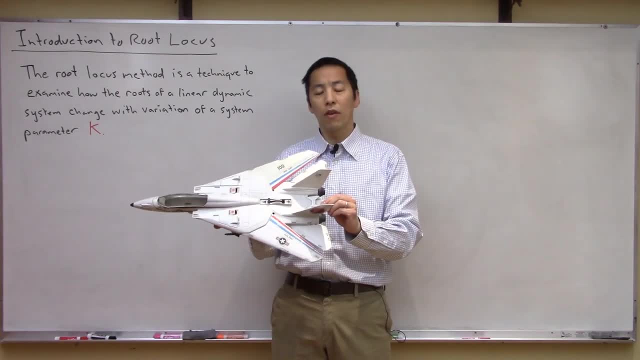 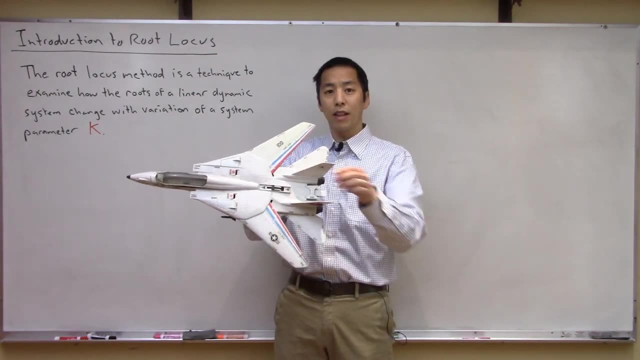 Now you might naturally ask yourself: well, what if I change this system in some fashion? For example, let's look at the wing sweep angle. What if I sweep the wings a little bit like that Now? does that change the endurance? 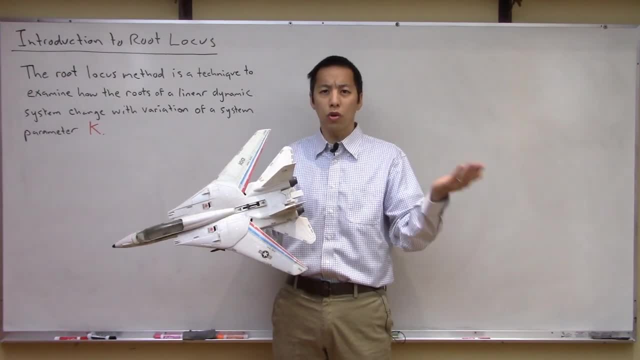 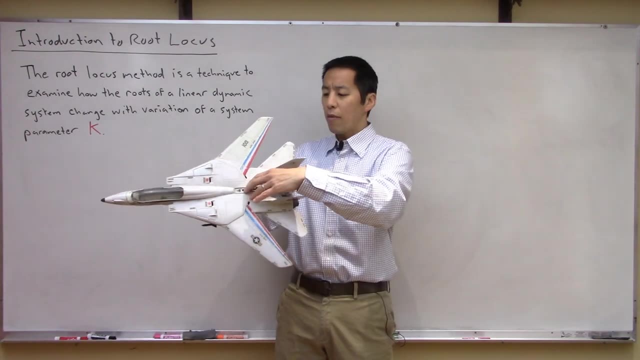 Can I stay in the air longer, shorter? You know who knows What, if I change this a little bit more? right, I sweep the wings a little more. Now, how did that change? How about, if I keep sweeping the wings all the way to you know, a little bit more? 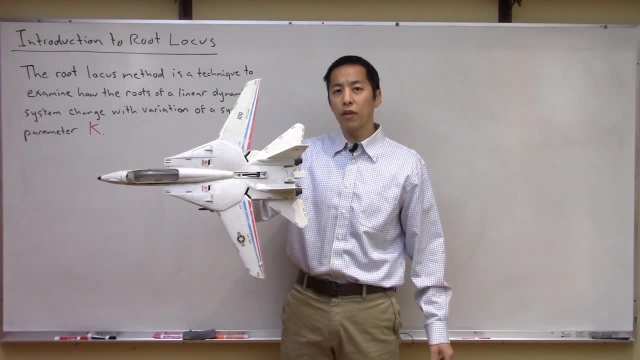 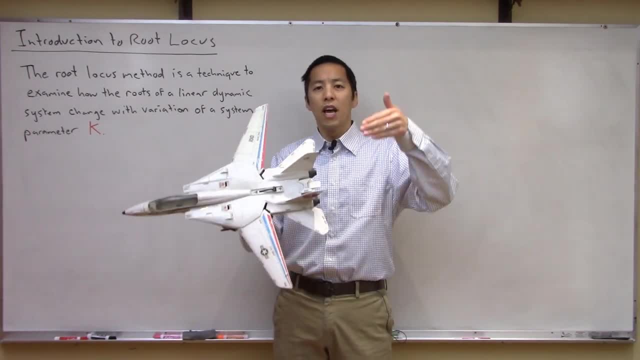 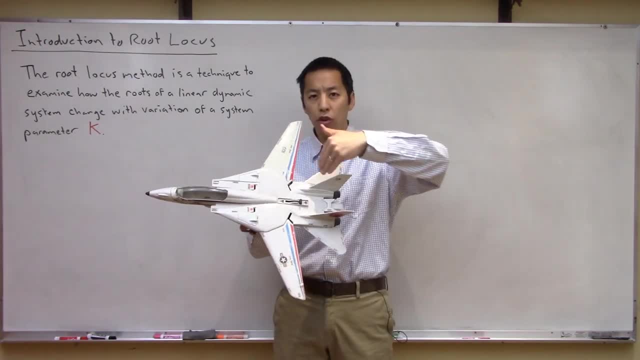 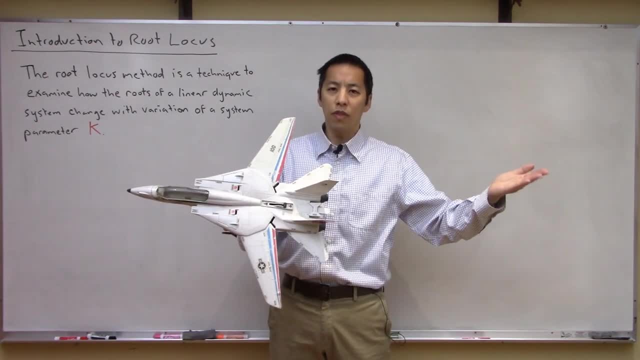 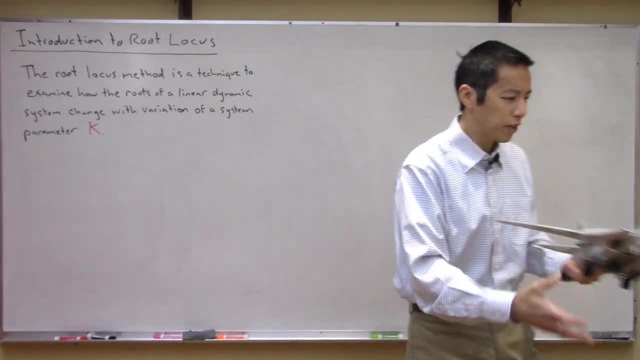 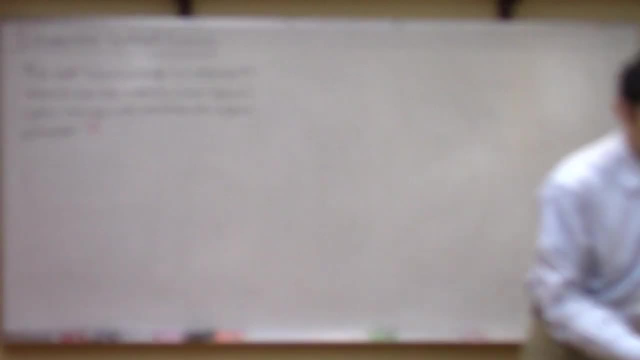 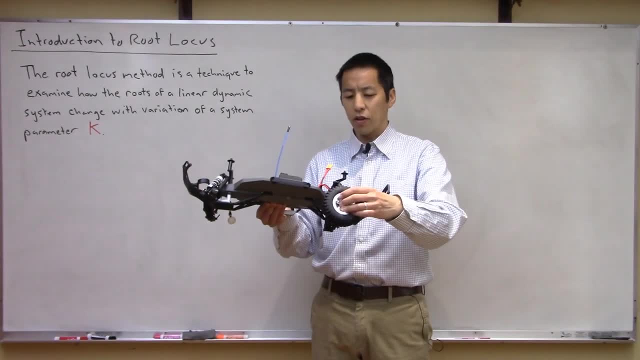 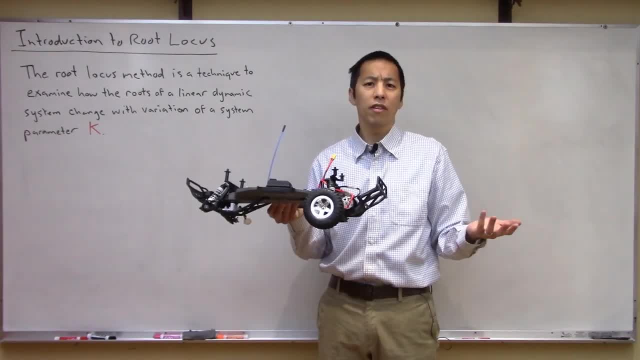 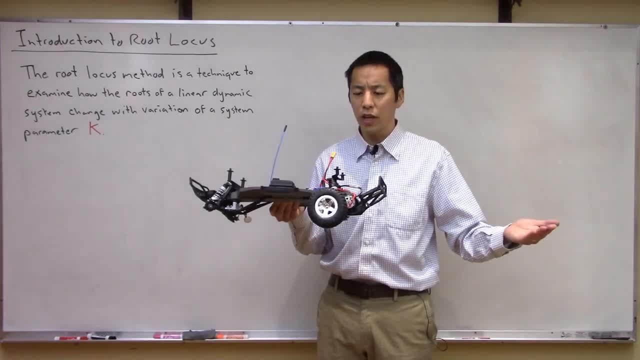 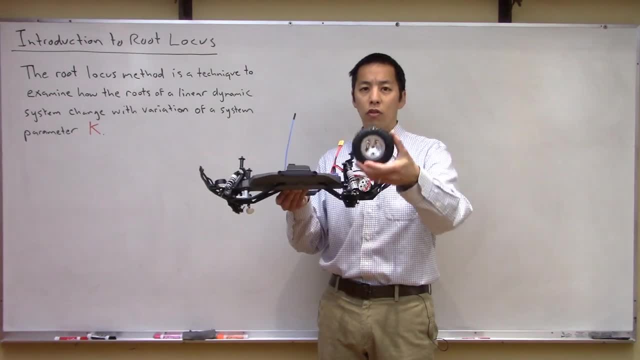 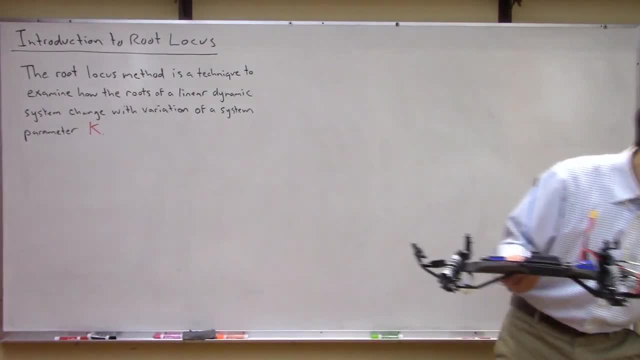 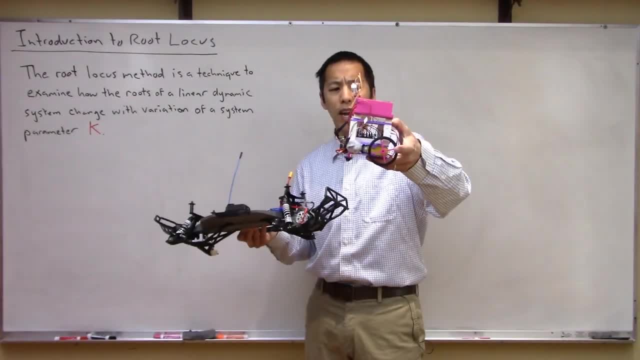 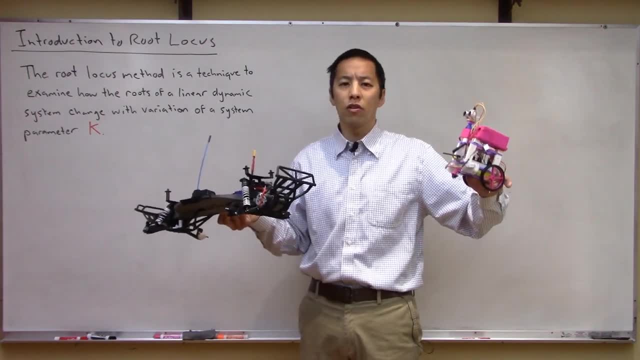 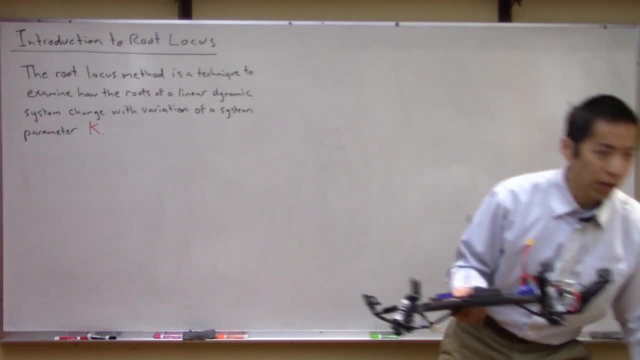 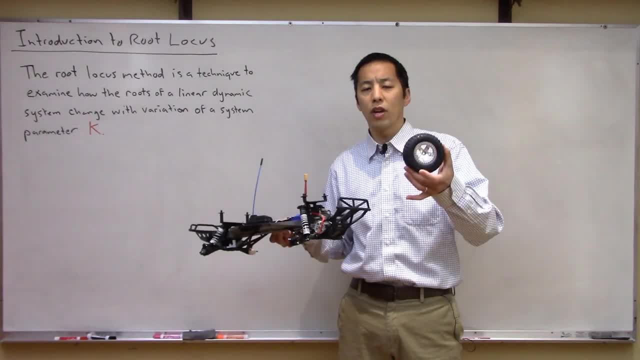 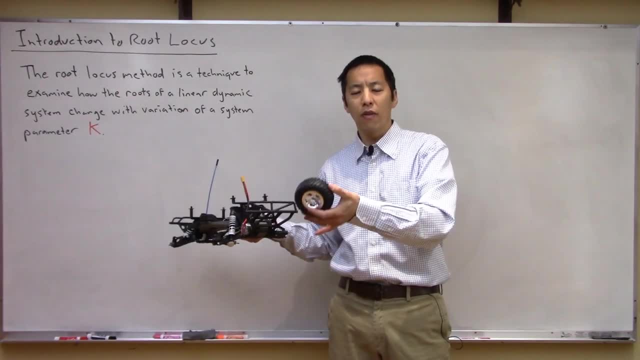 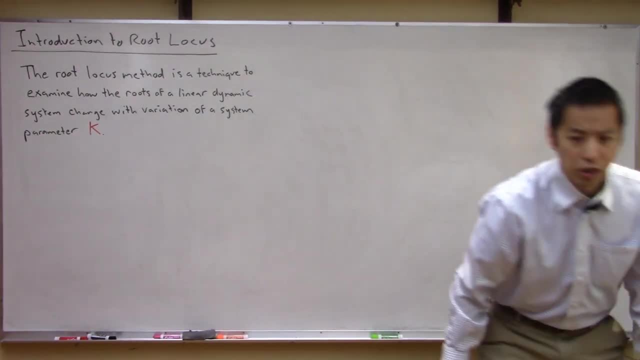 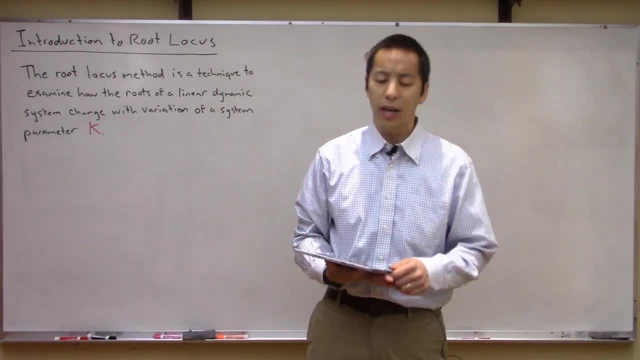 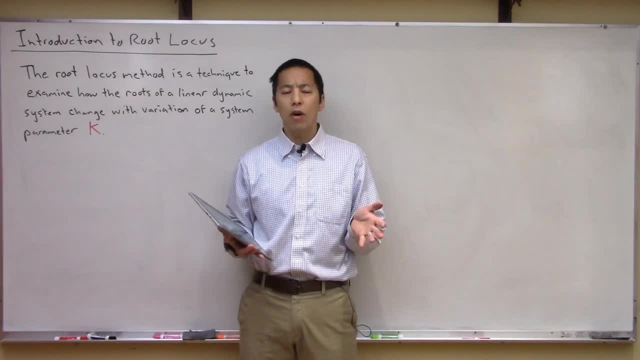 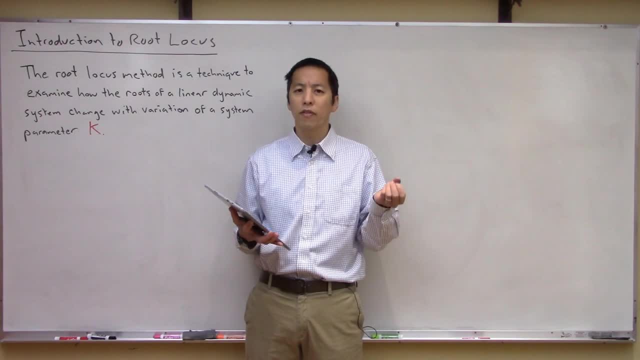 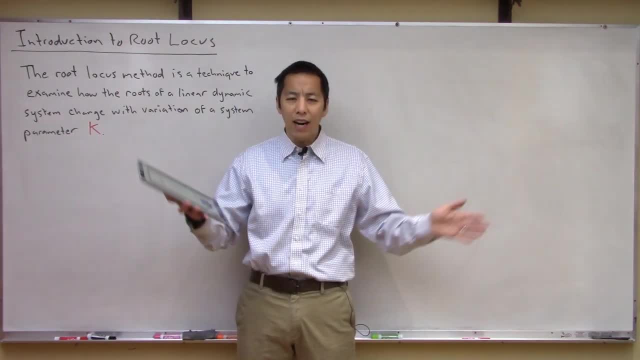 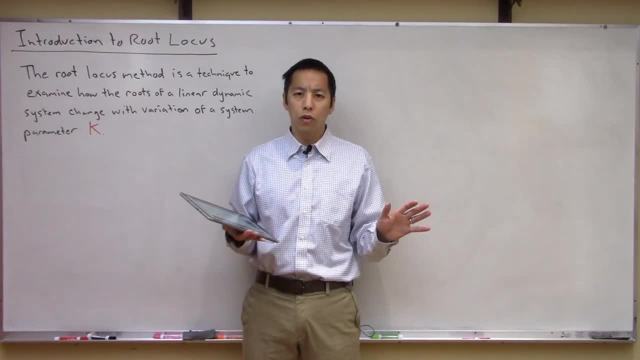 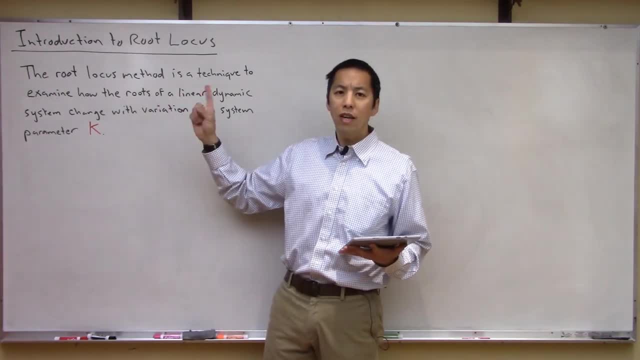 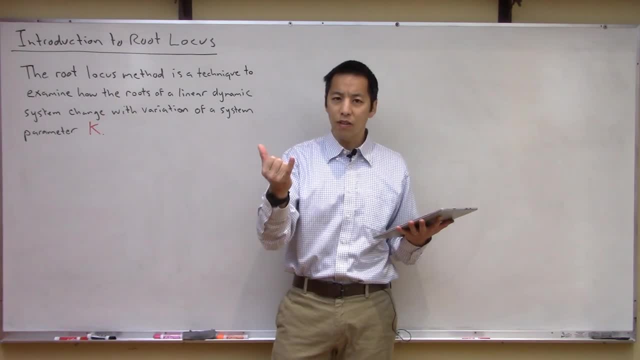 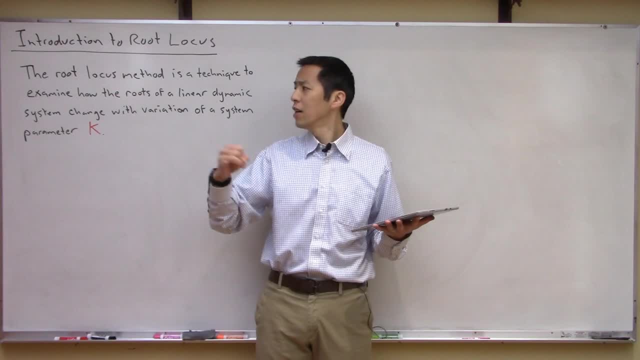 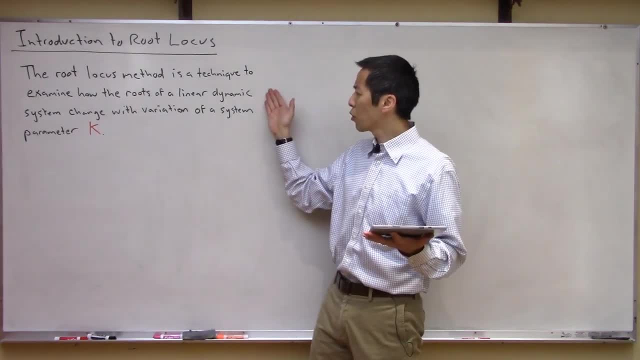 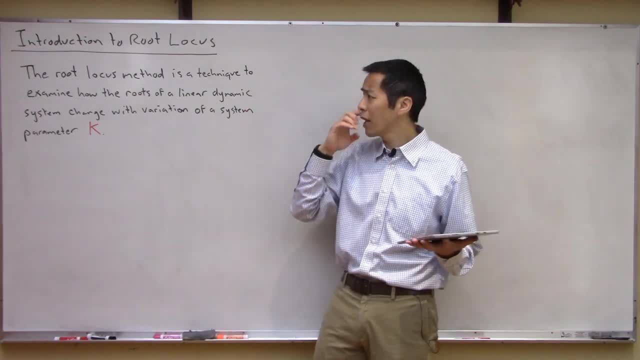 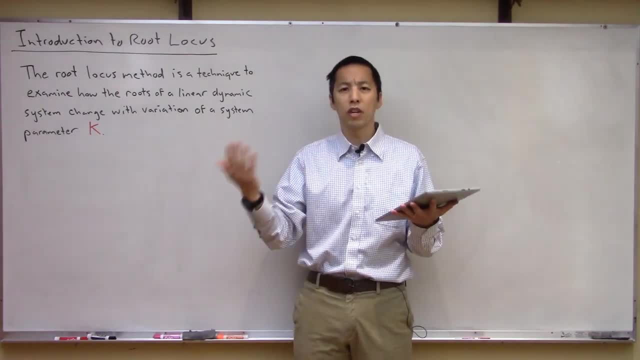 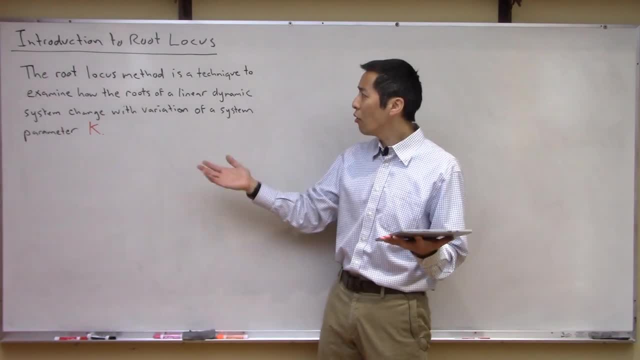 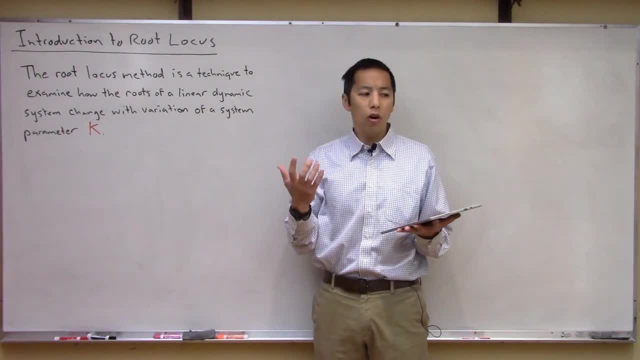 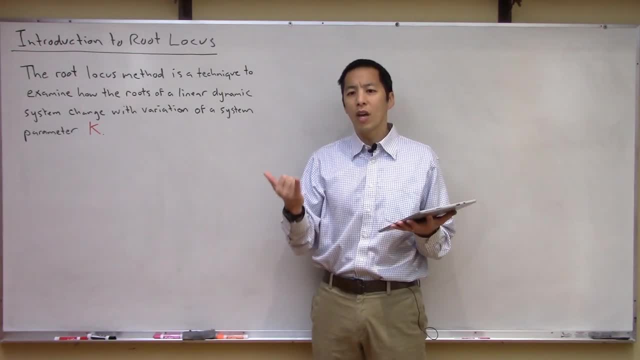 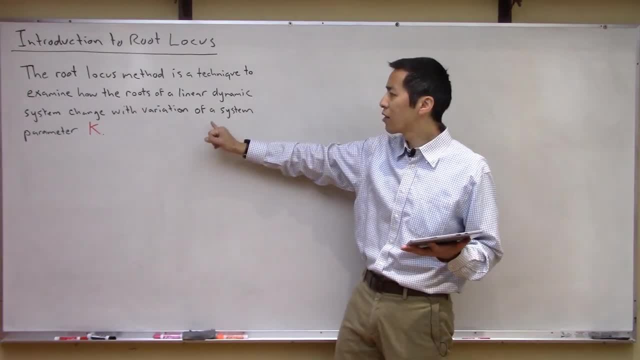 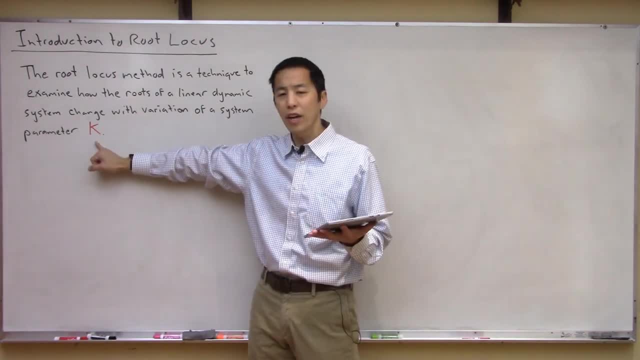 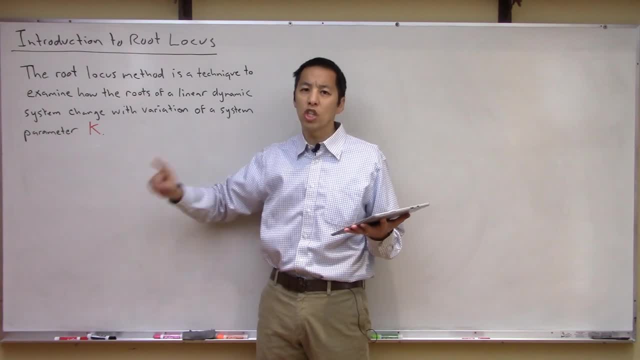 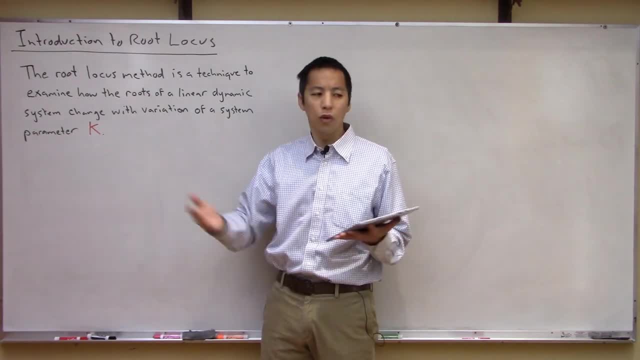 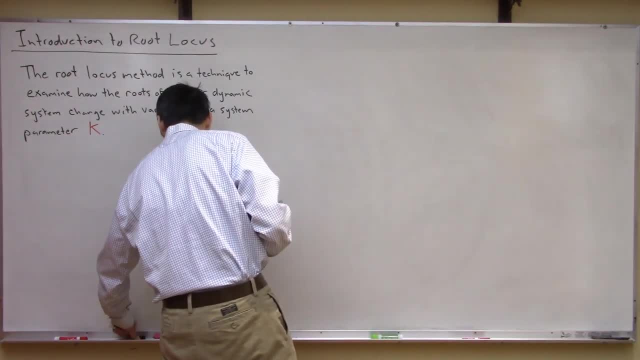 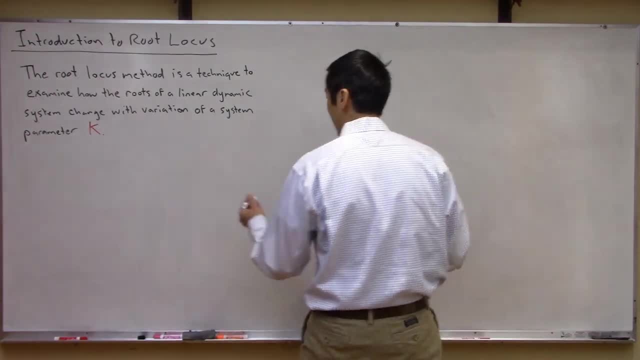 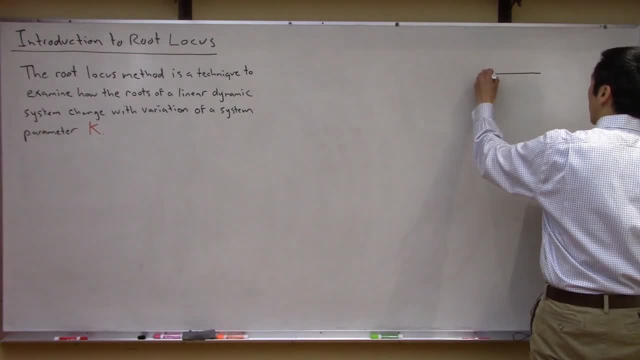 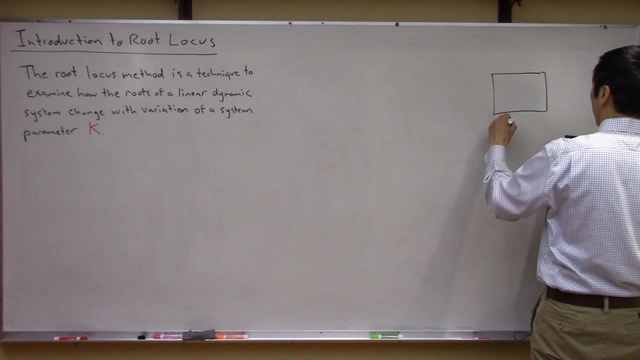 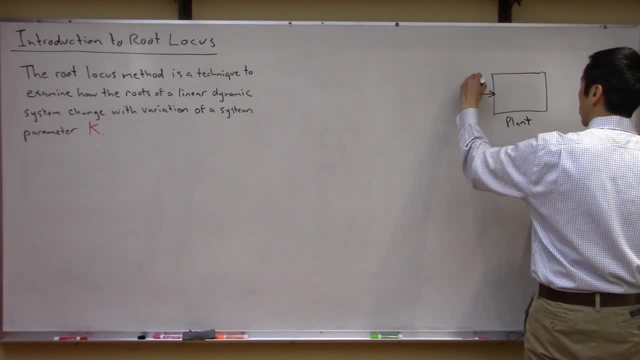 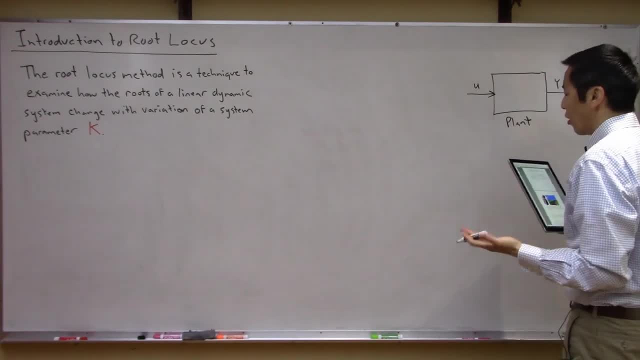 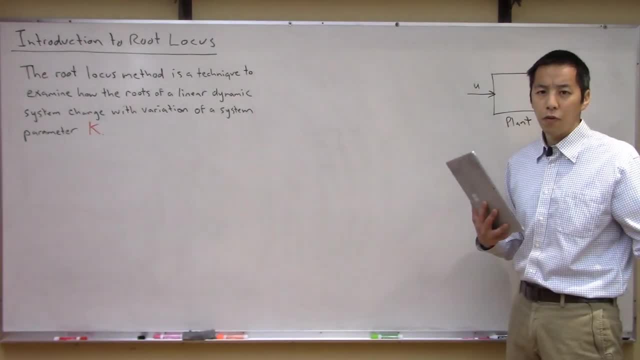 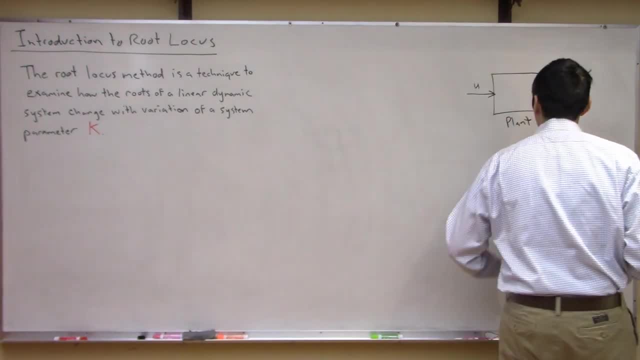 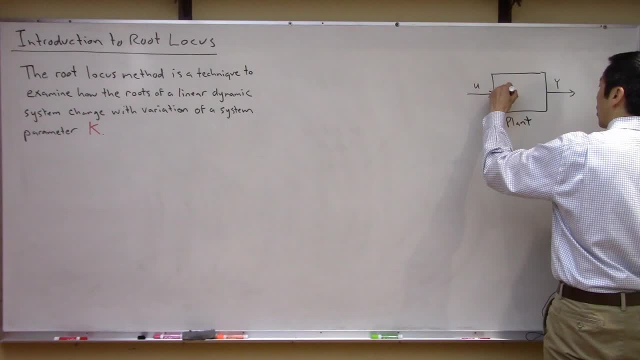 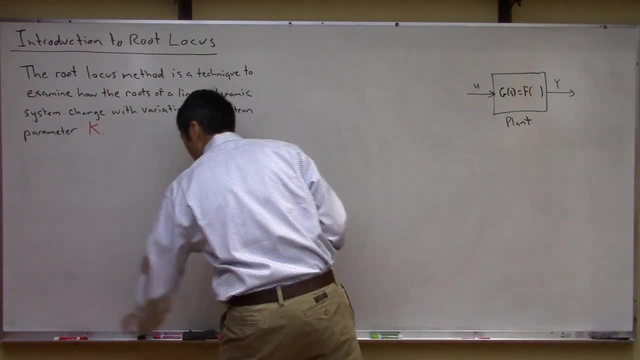 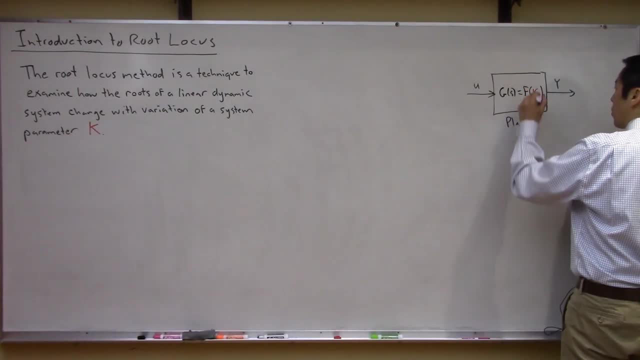 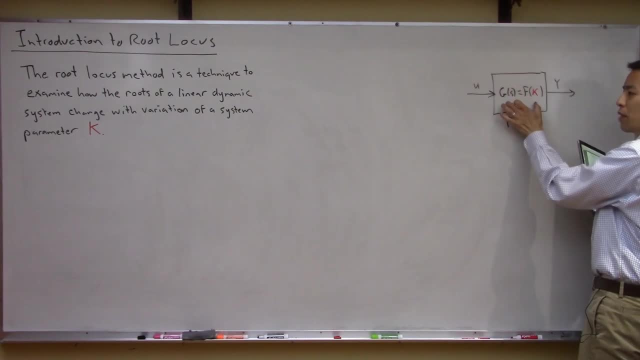 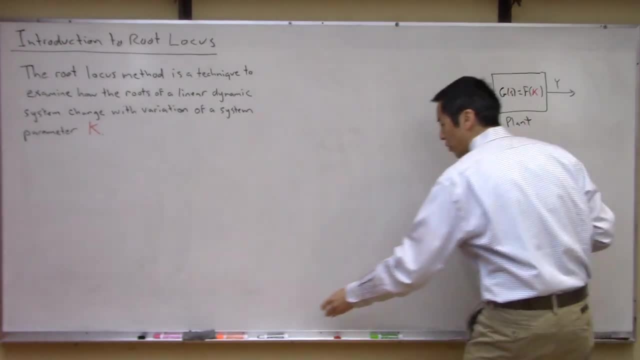 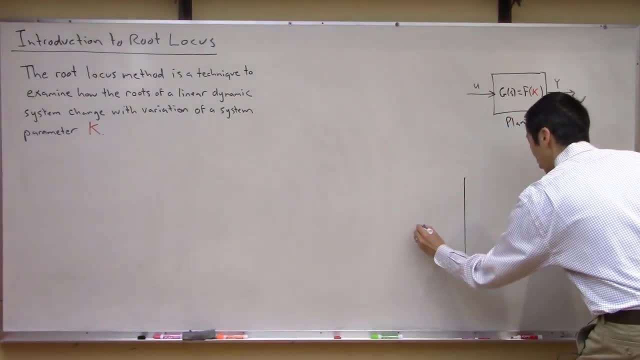 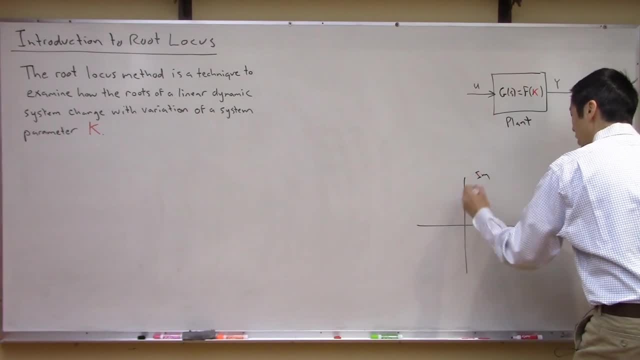 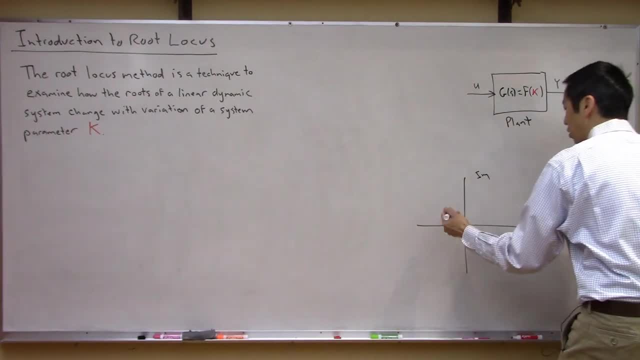 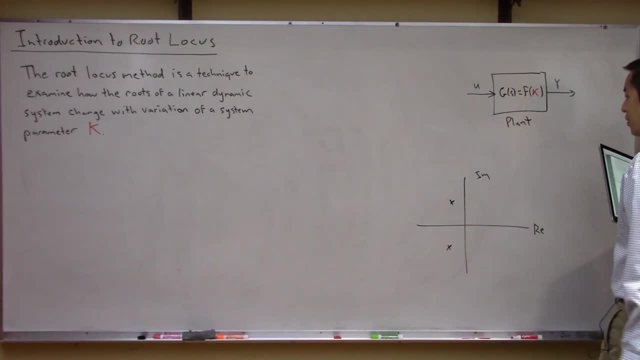 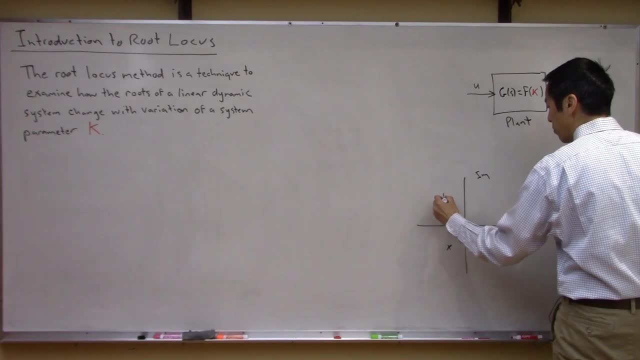 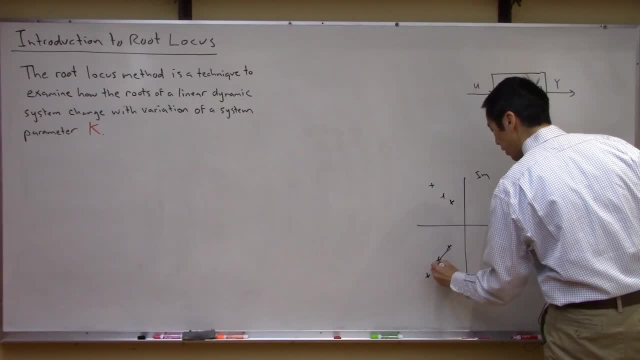 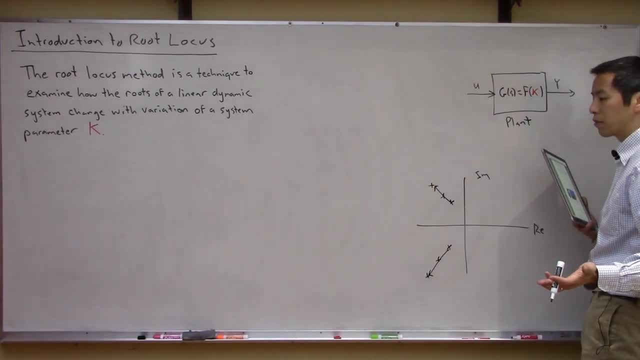 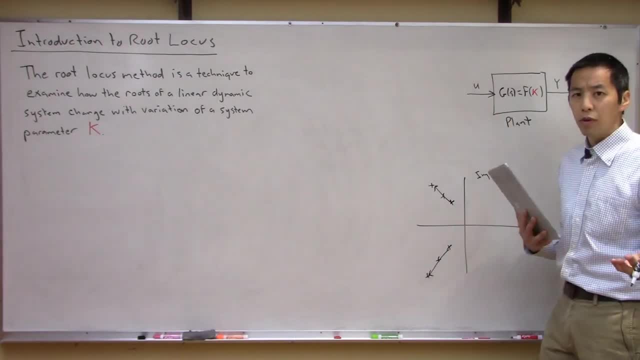 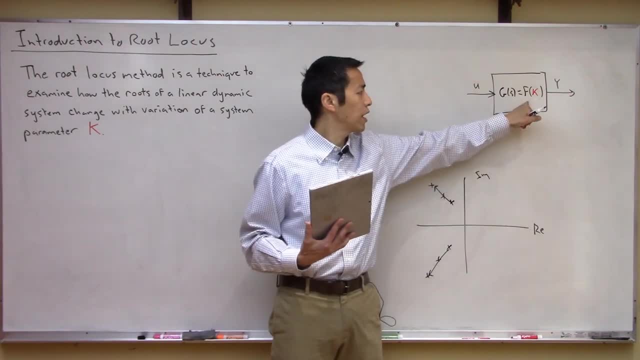 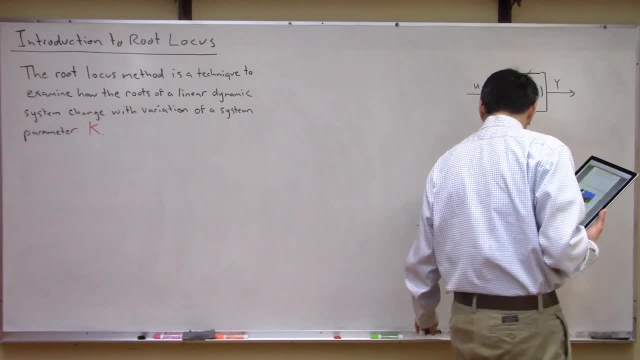 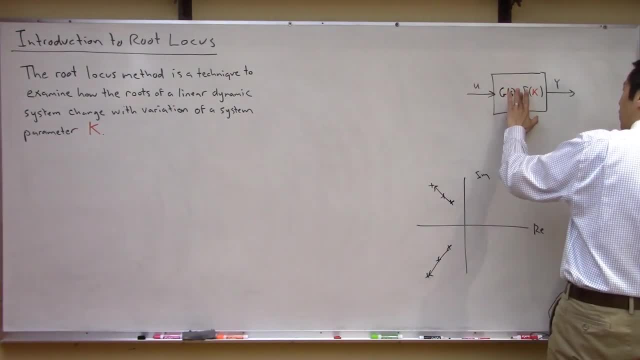 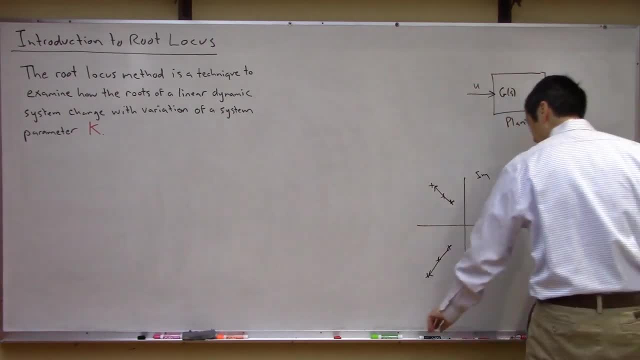 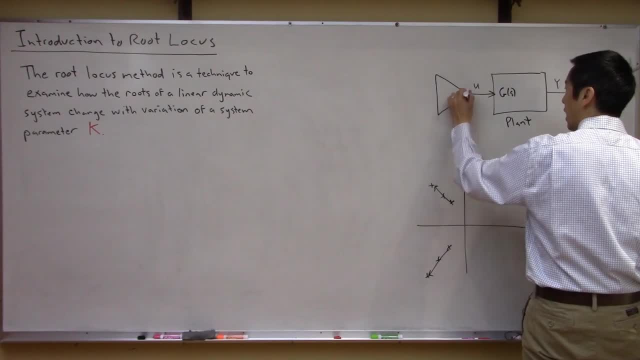 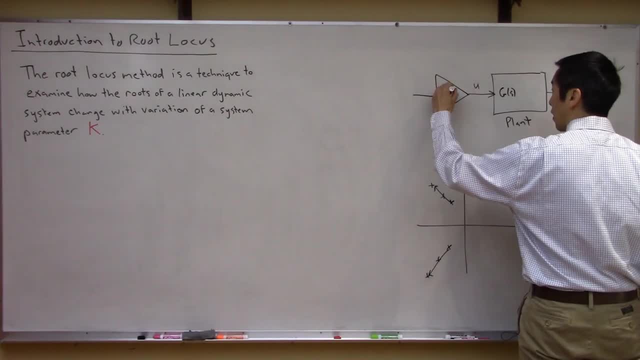 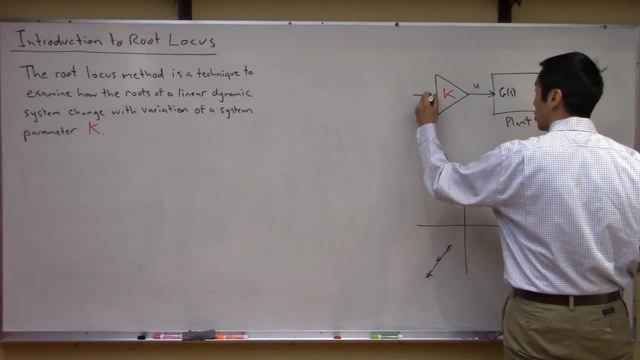 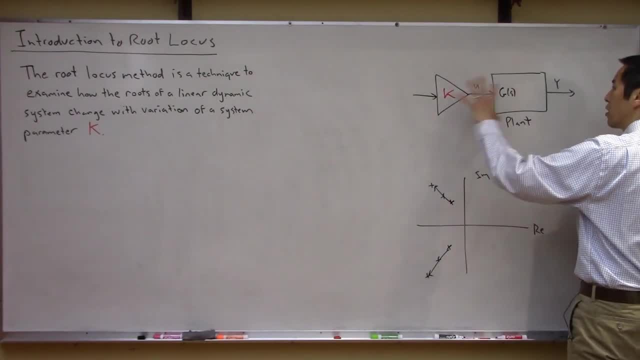 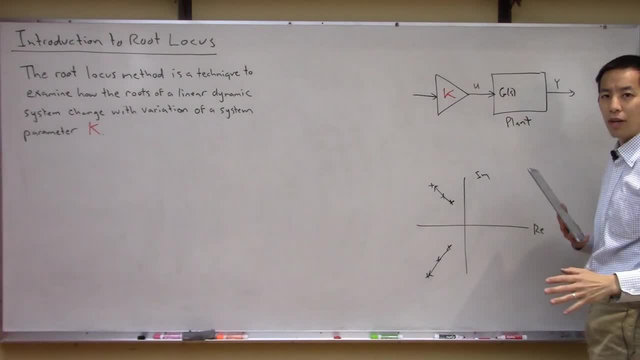 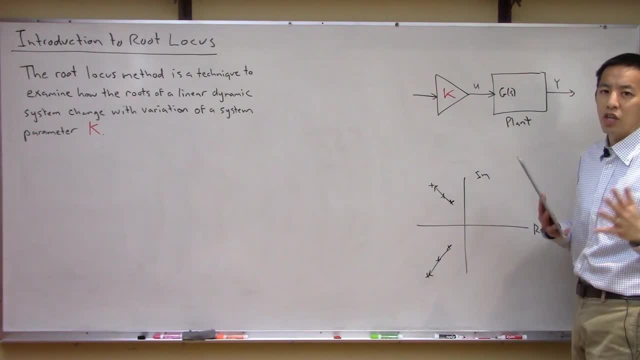 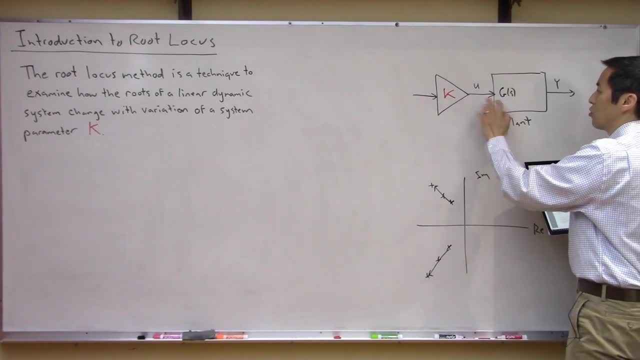 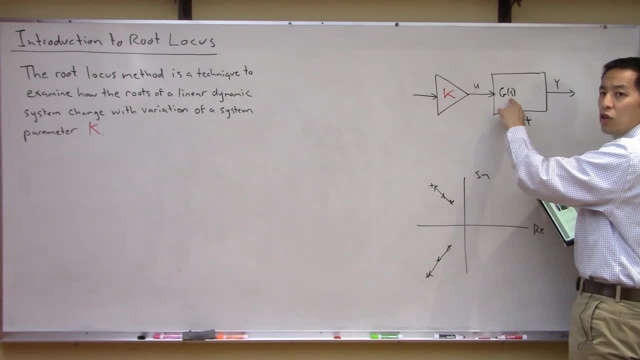 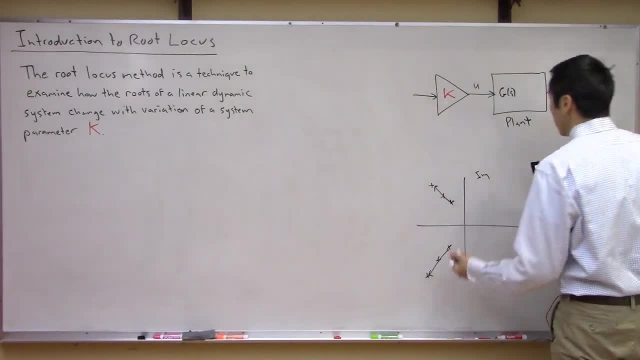 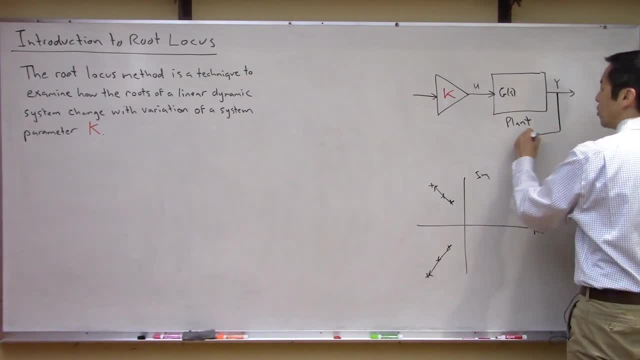 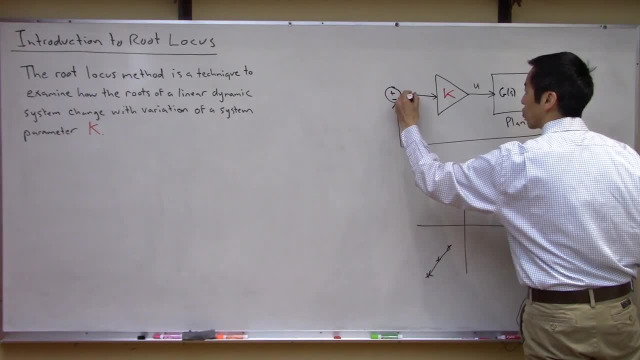 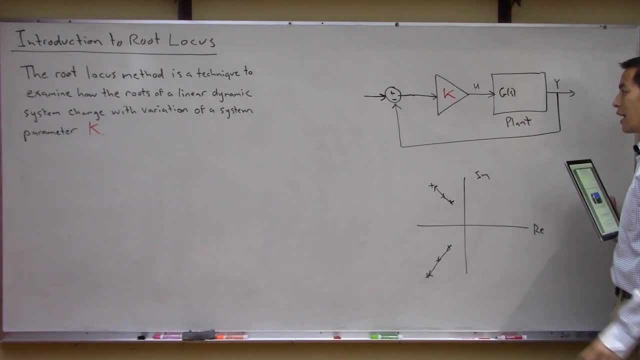 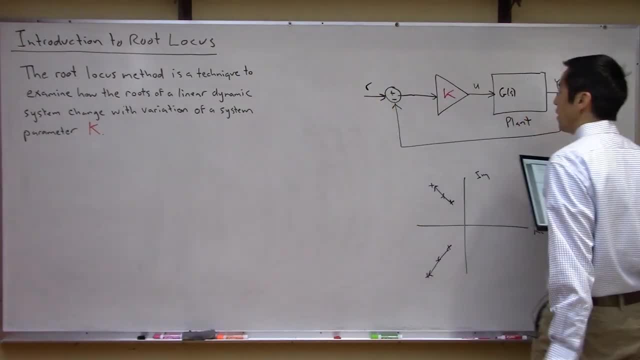 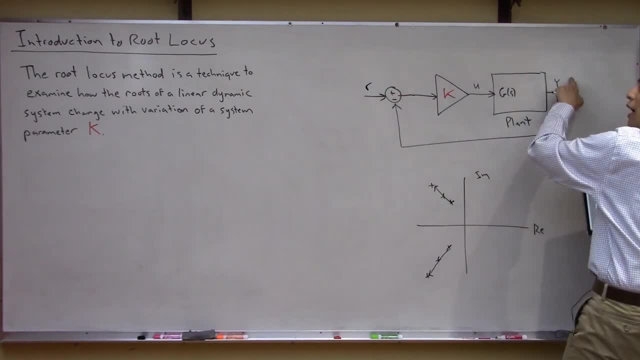 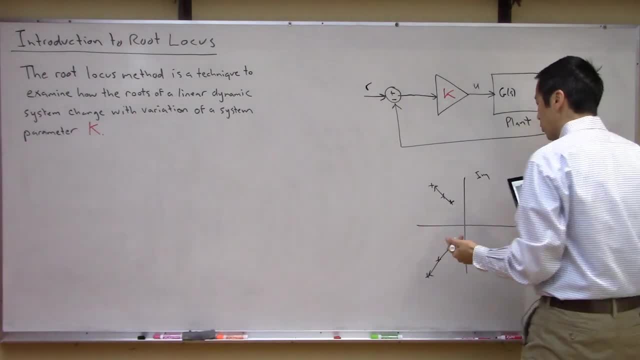 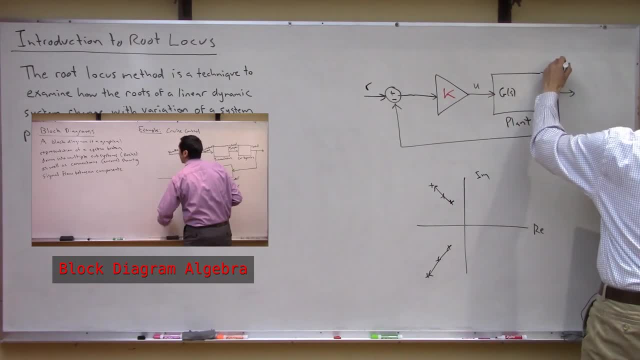 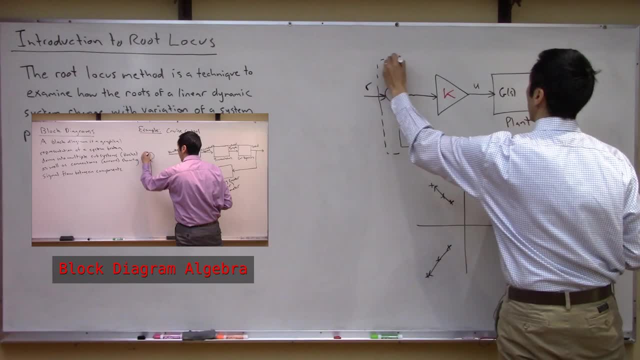 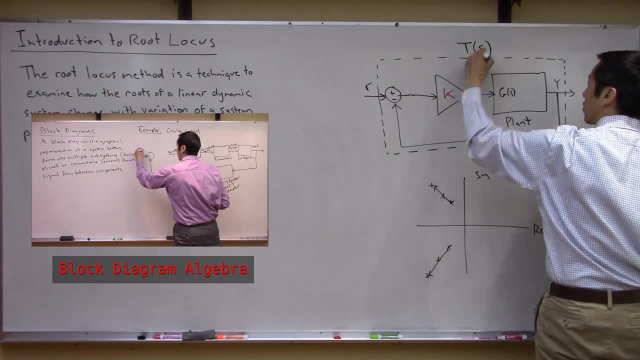 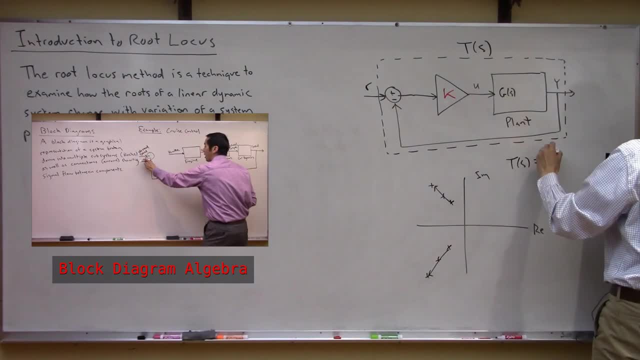 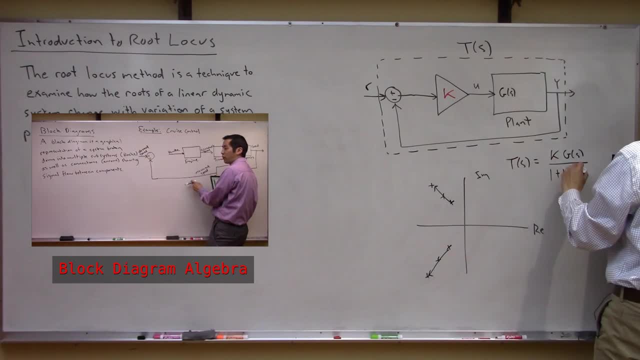 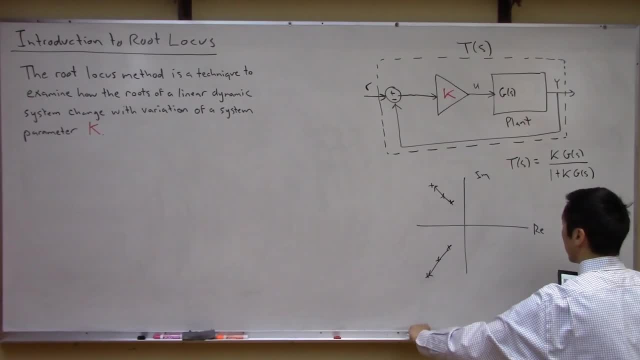 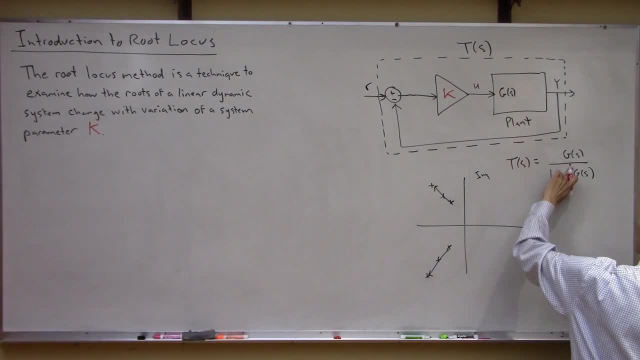 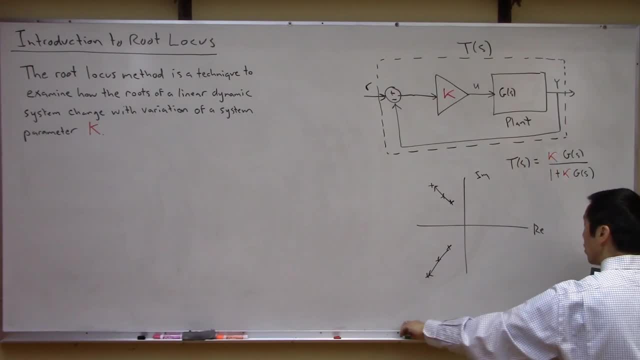 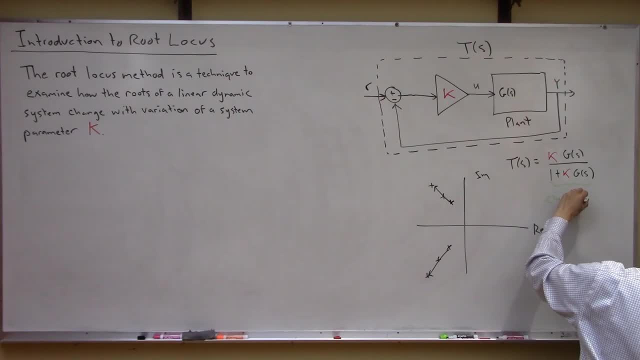 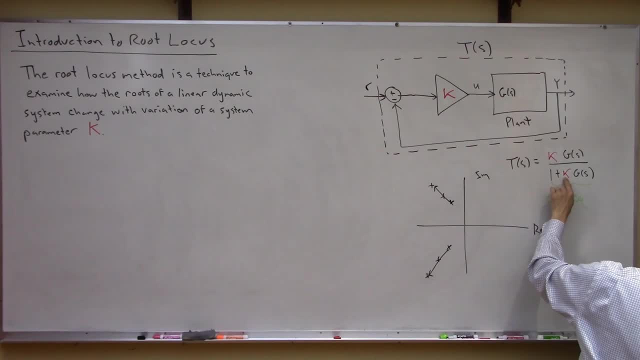 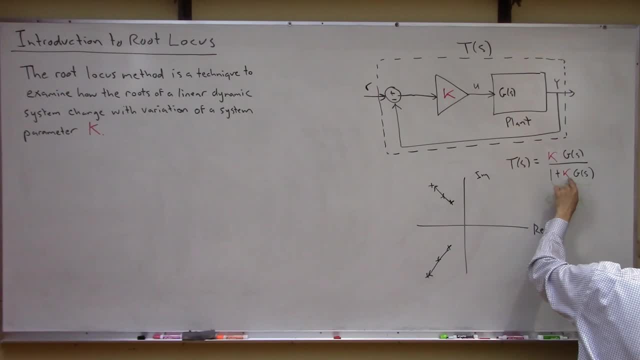 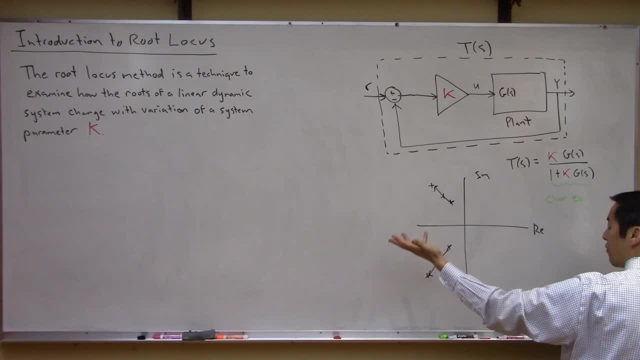 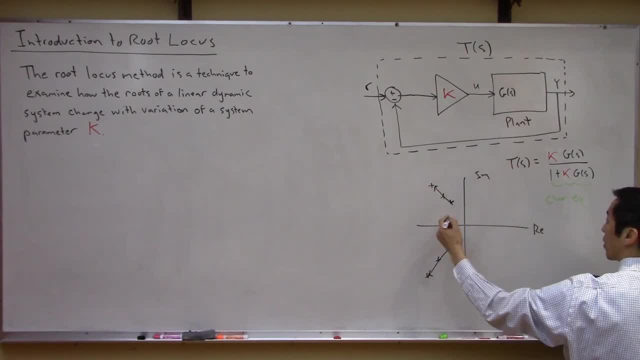 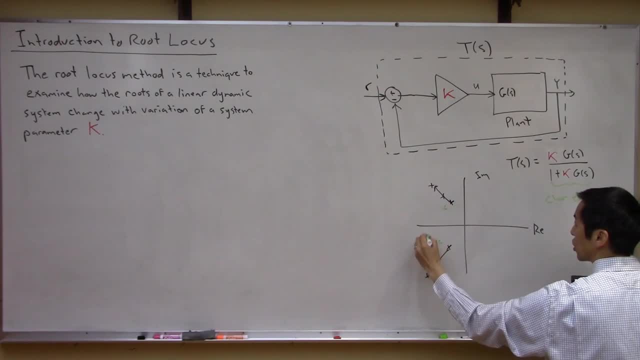 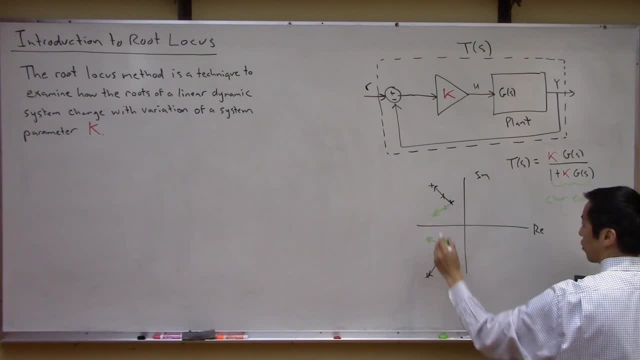 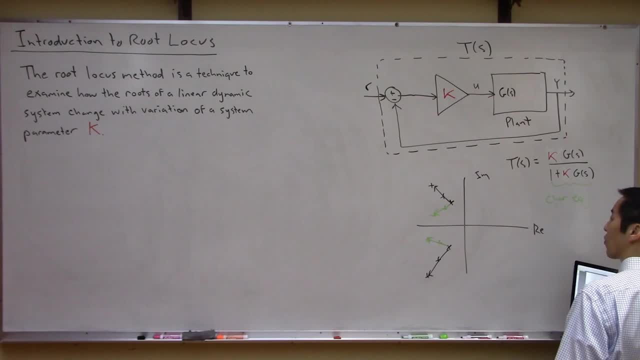 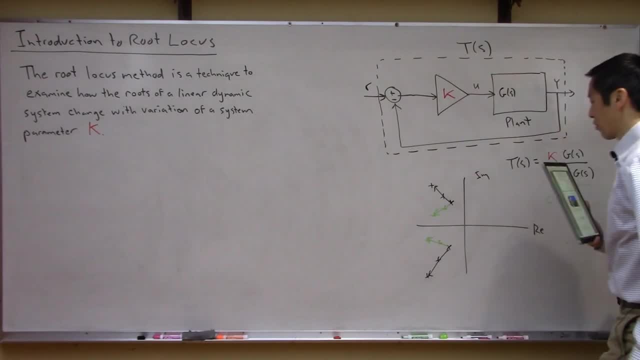 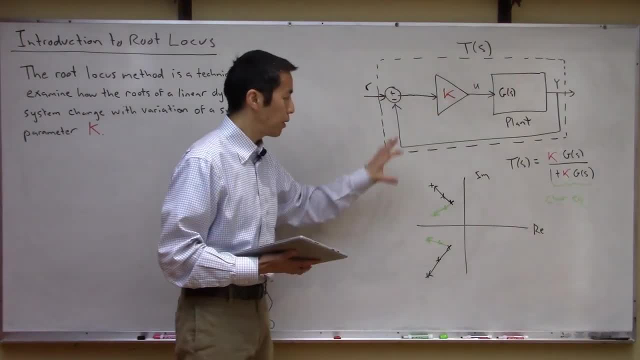 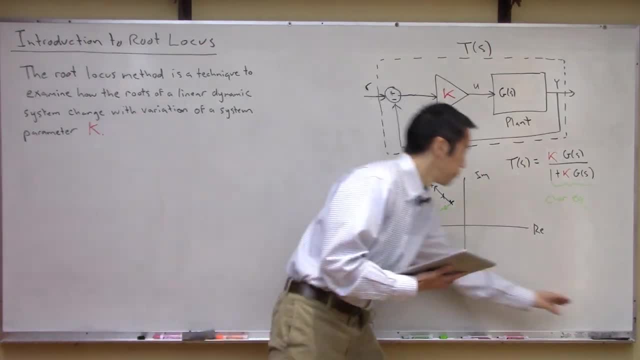 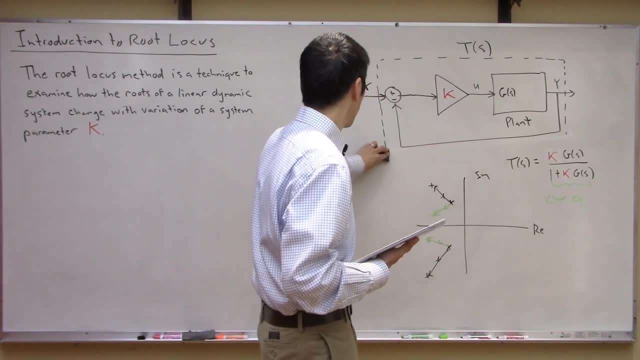 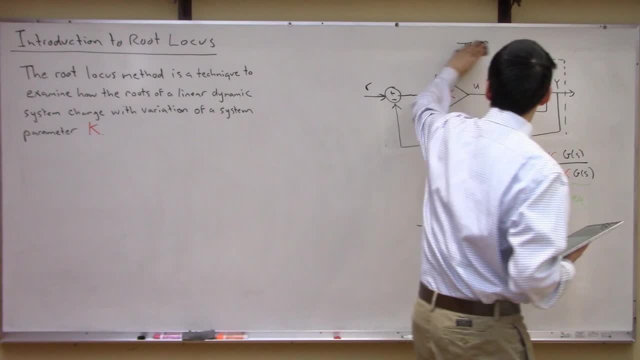 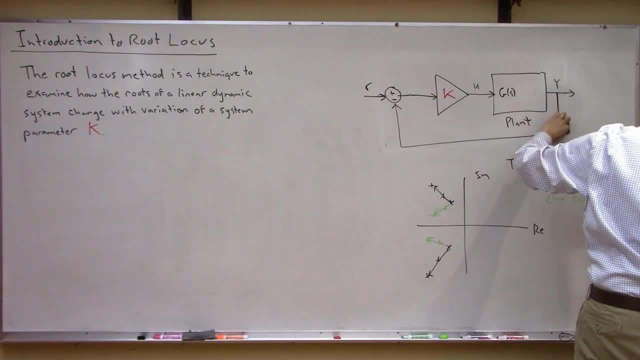 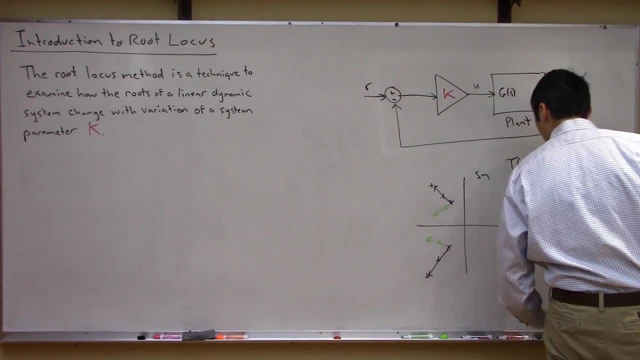 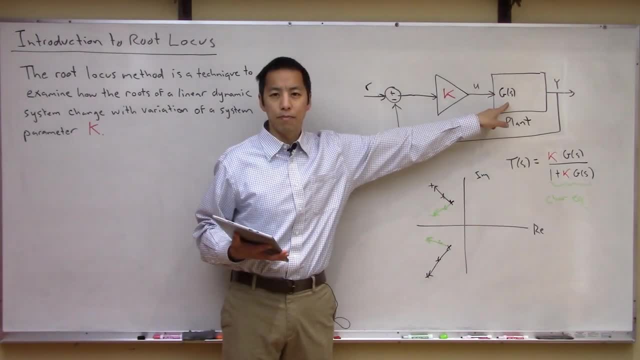 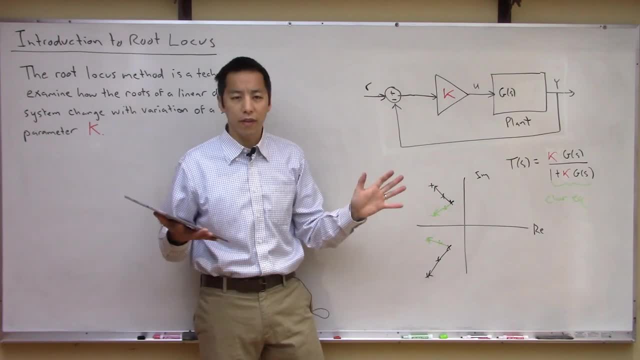 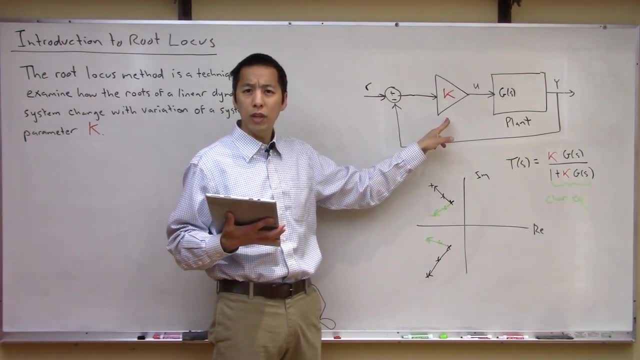 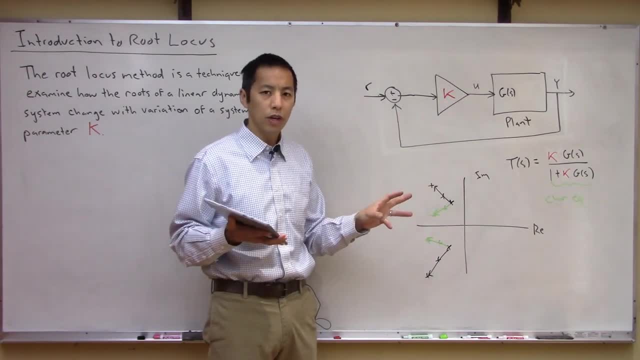 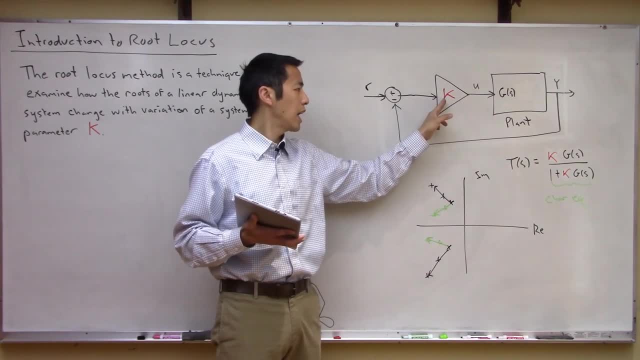 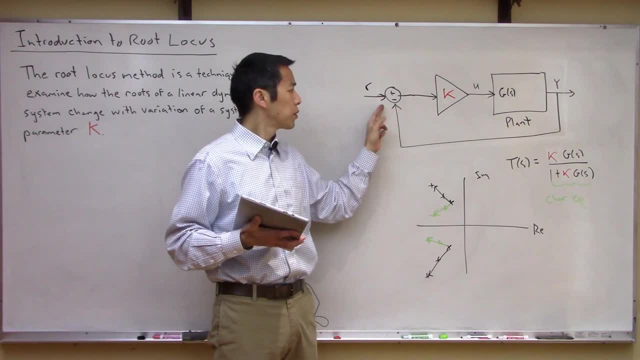 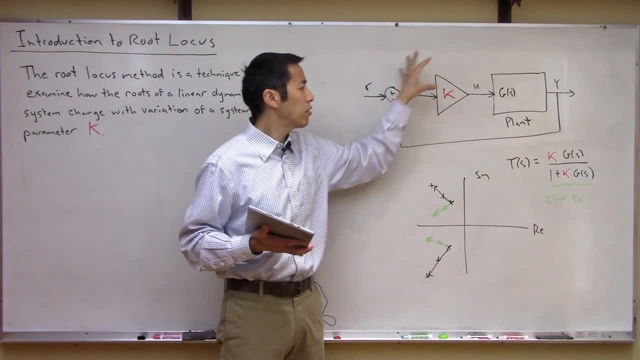 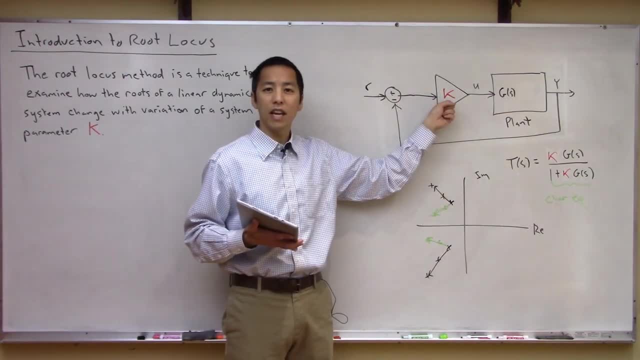 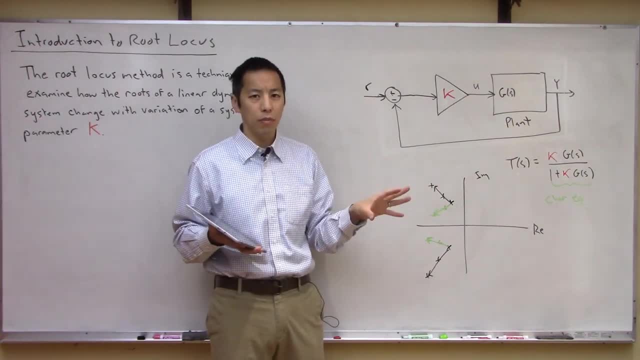 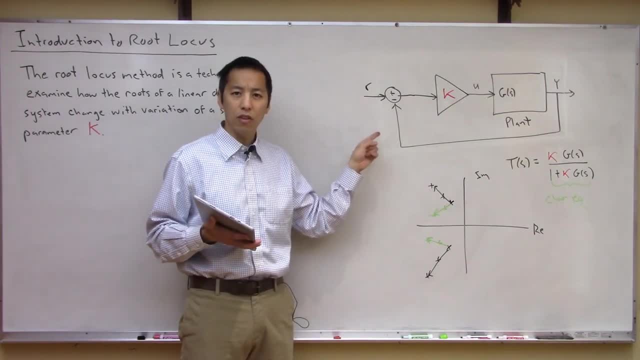 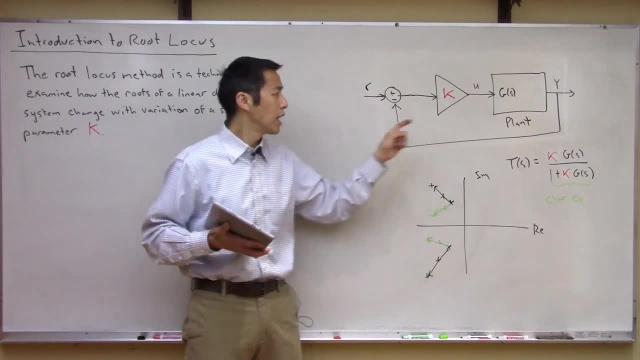 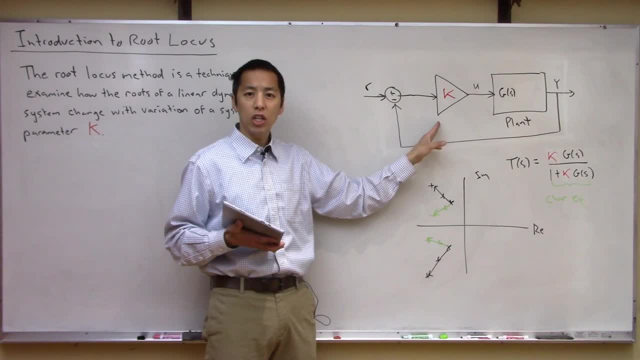 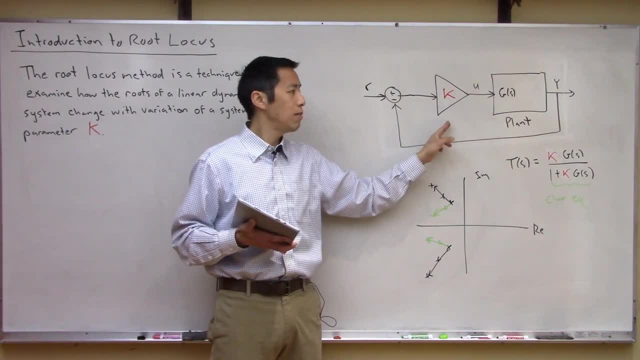 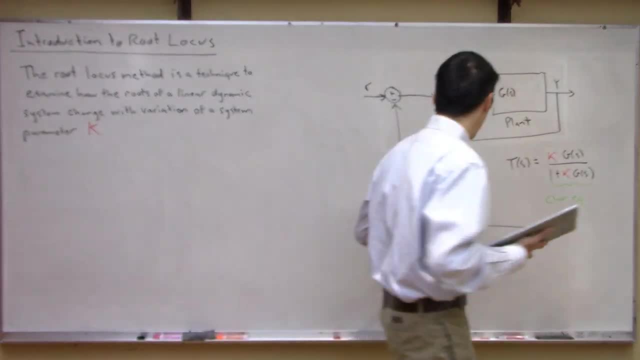 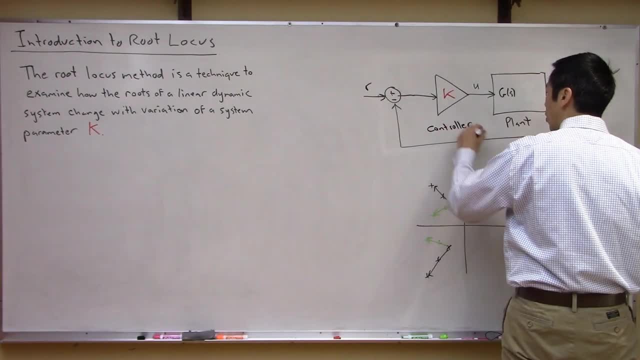 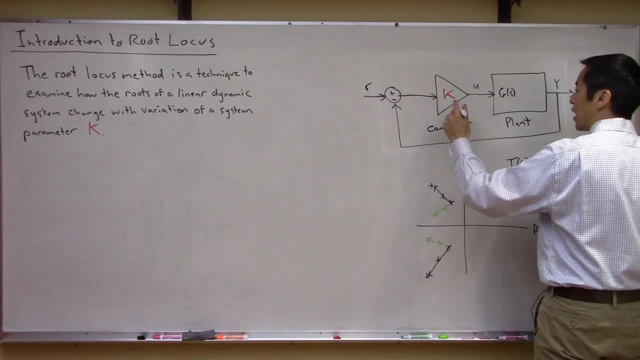 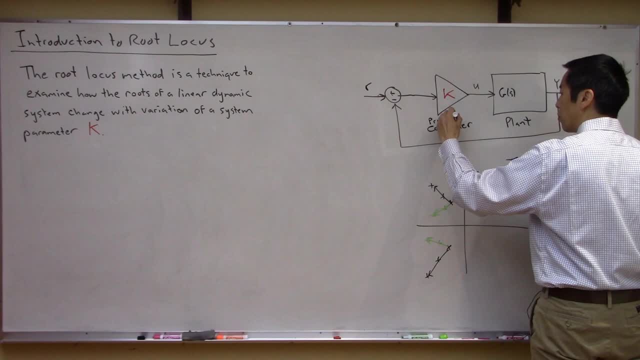 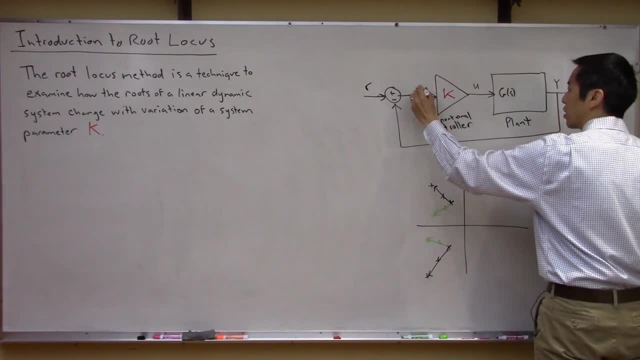 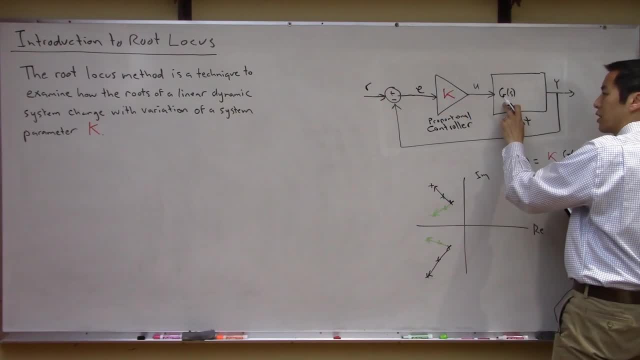 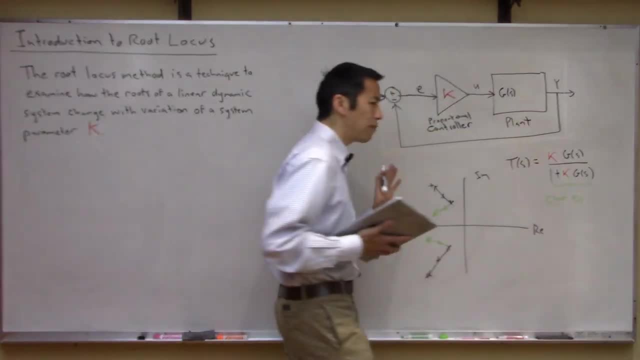 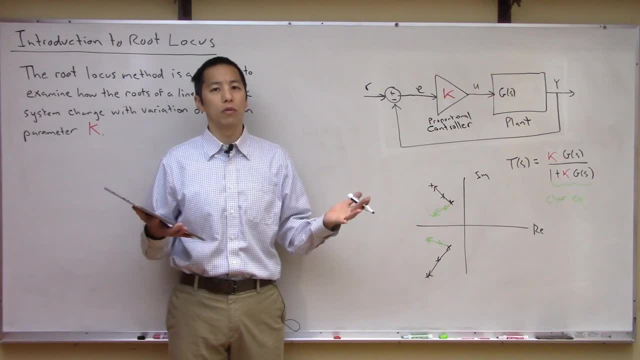 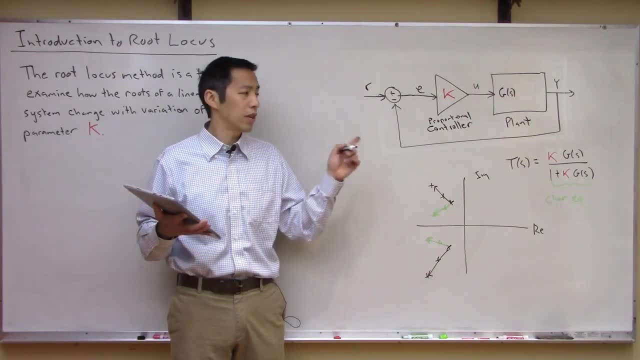 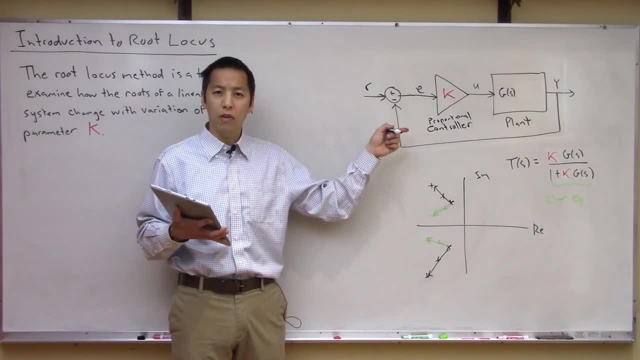 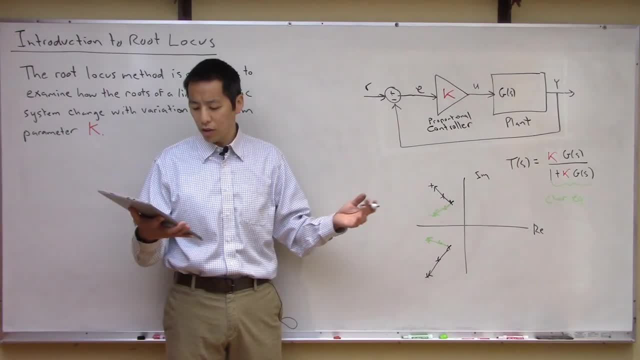 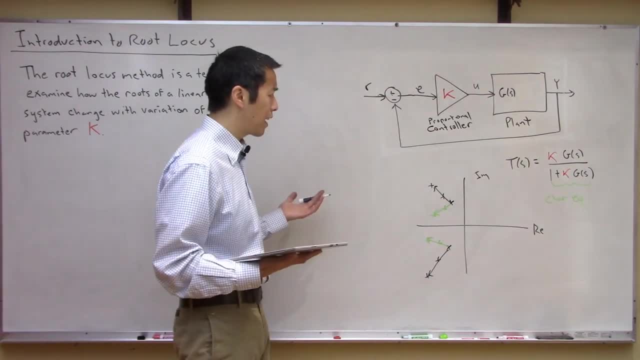 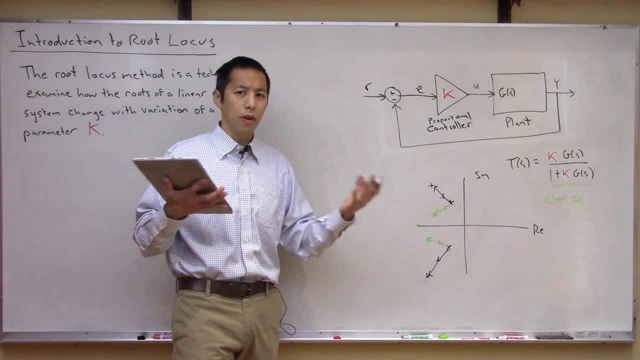 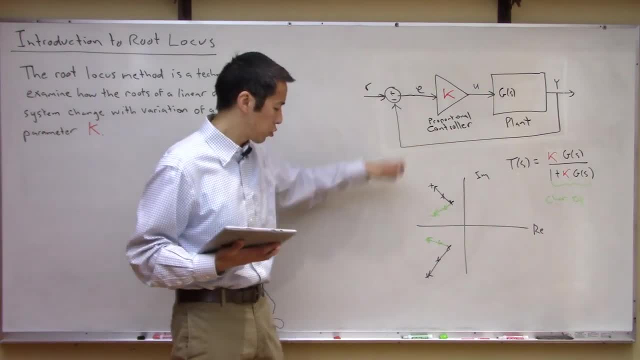 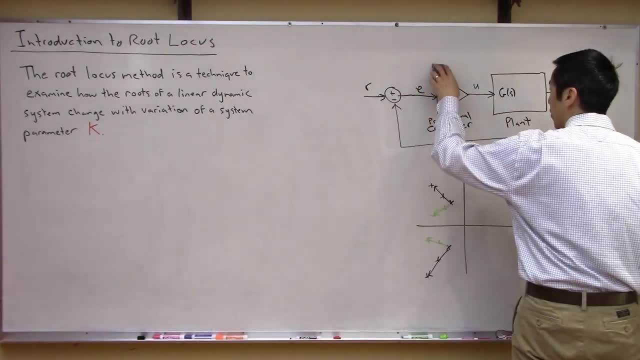 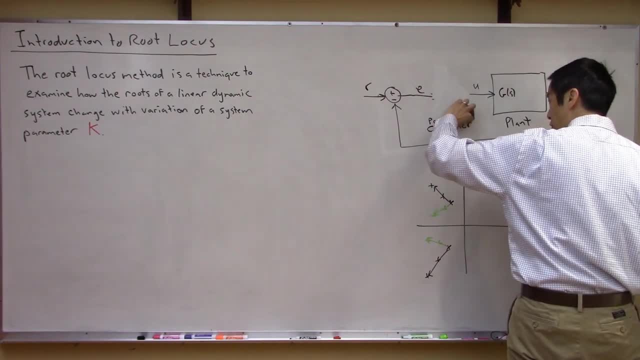 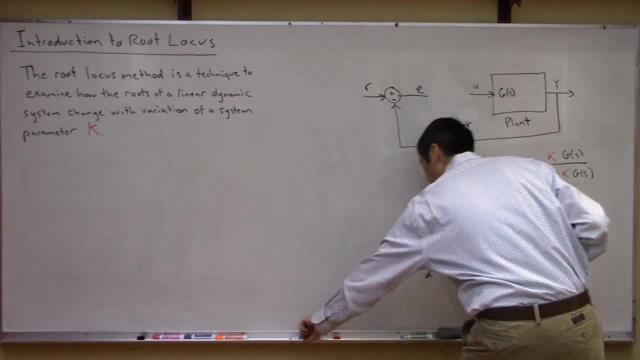 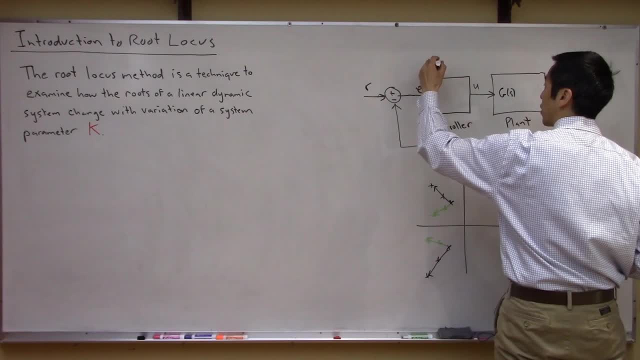 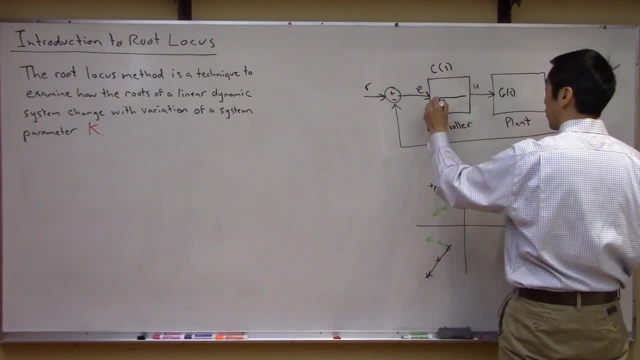 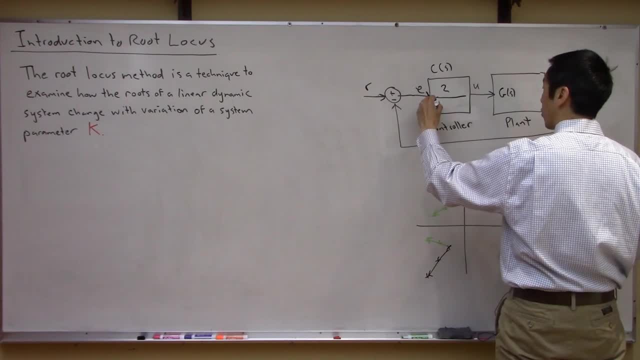 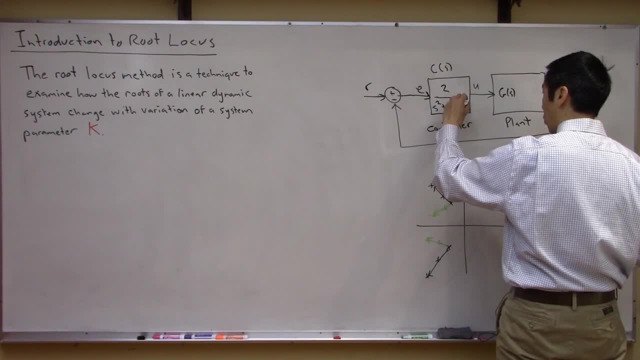 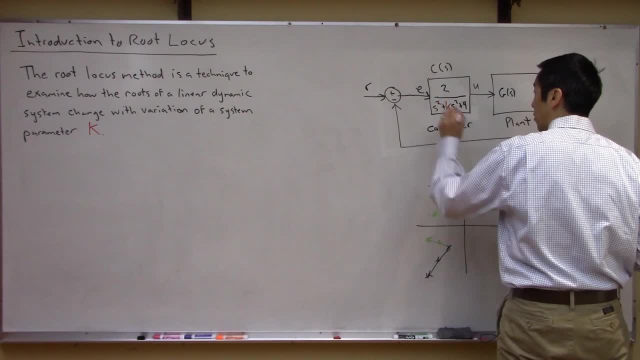 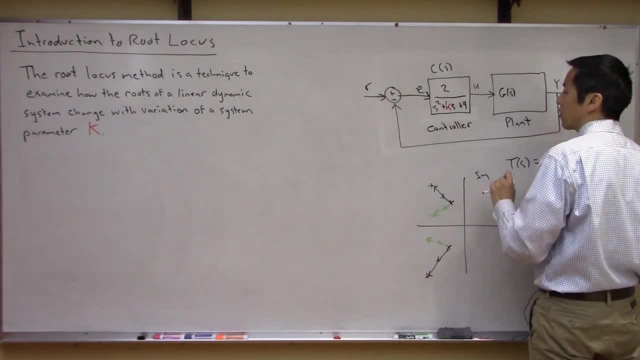 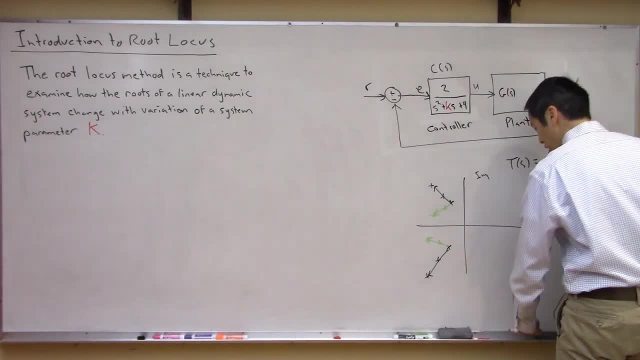 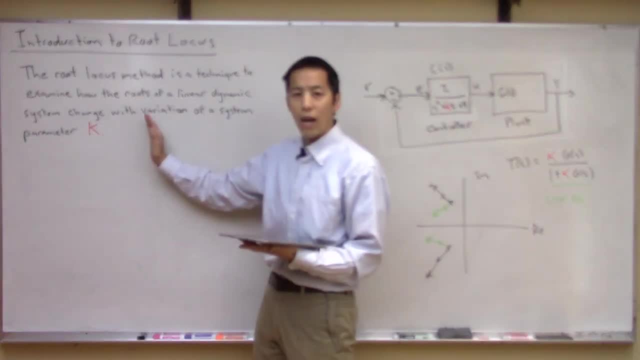 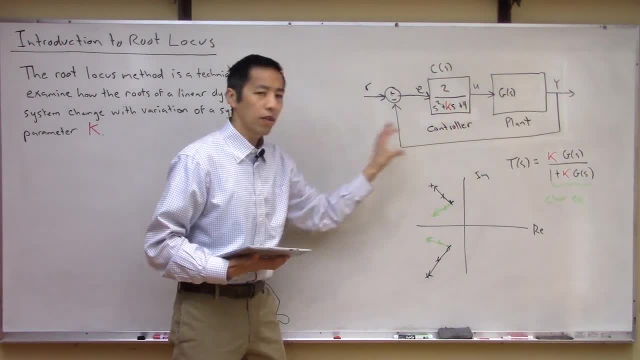 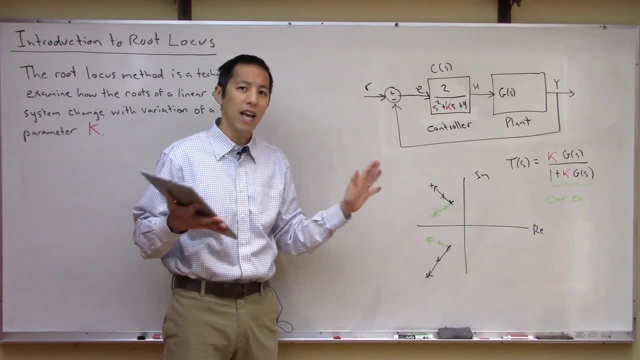 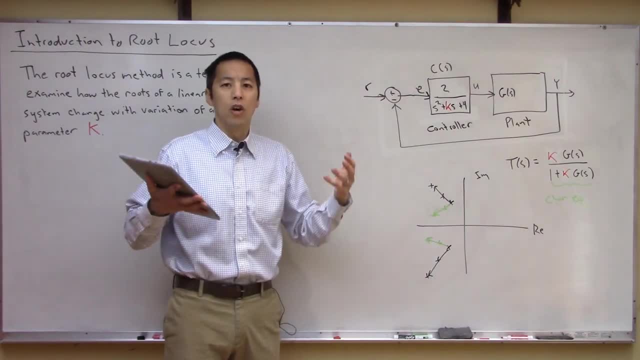 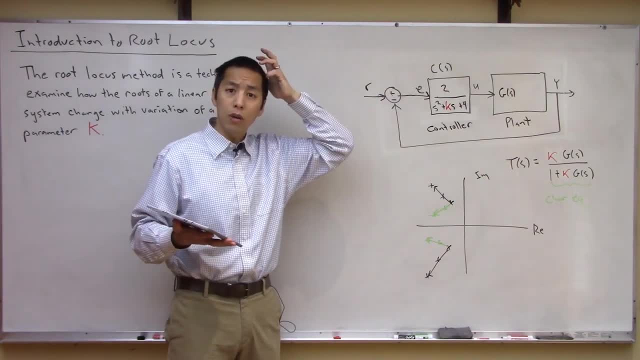 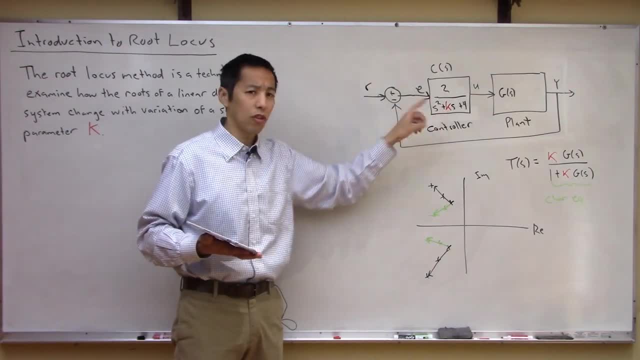 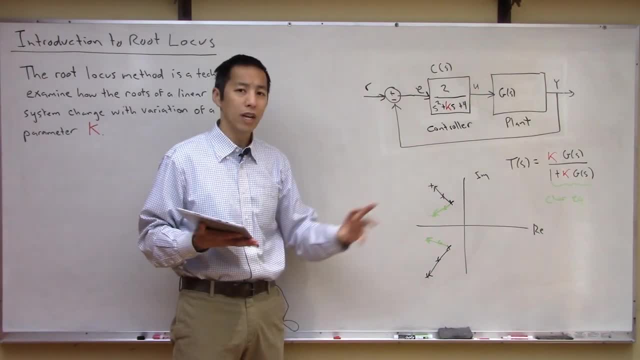 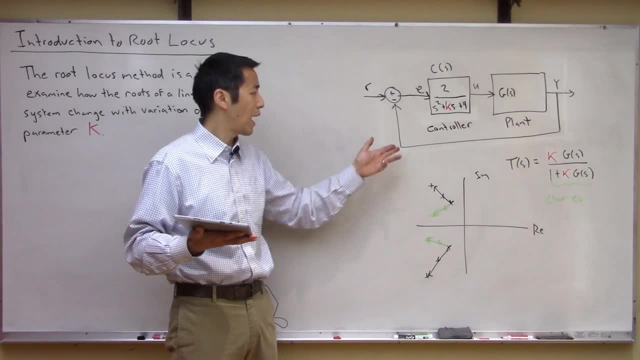 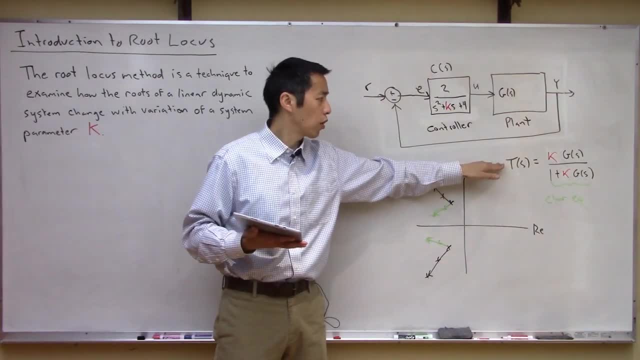 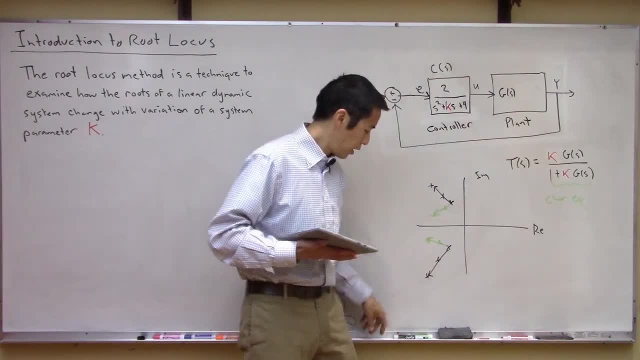 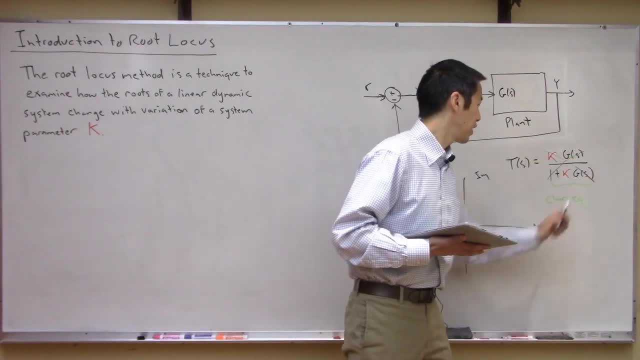 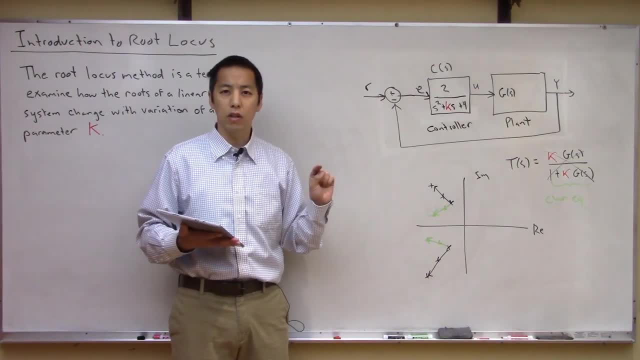 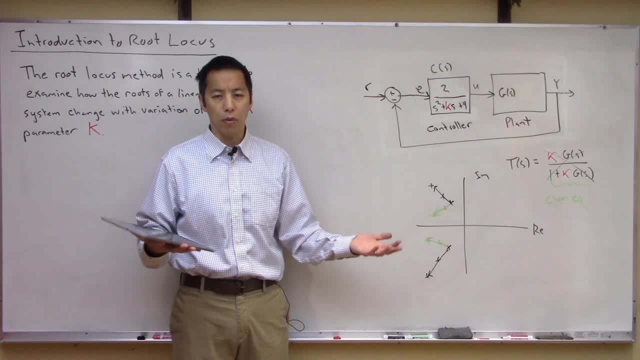 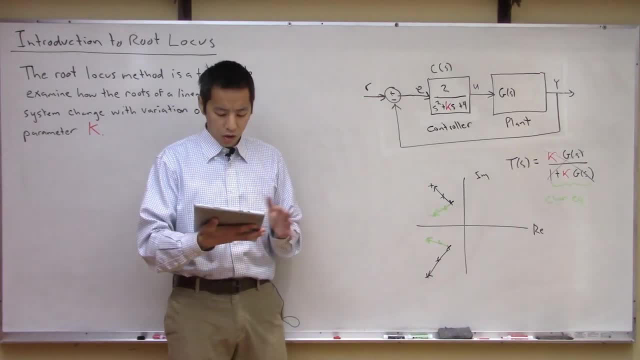 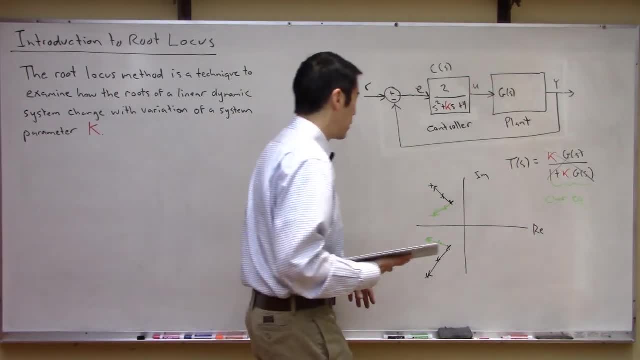 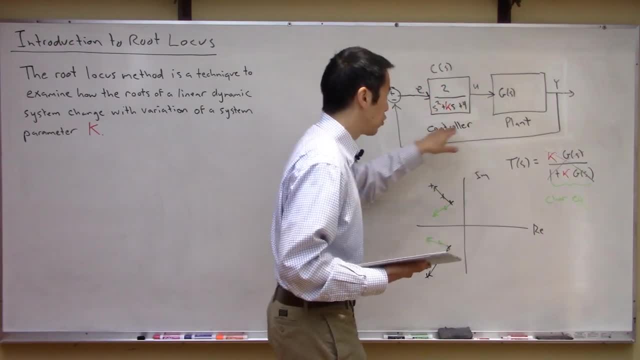 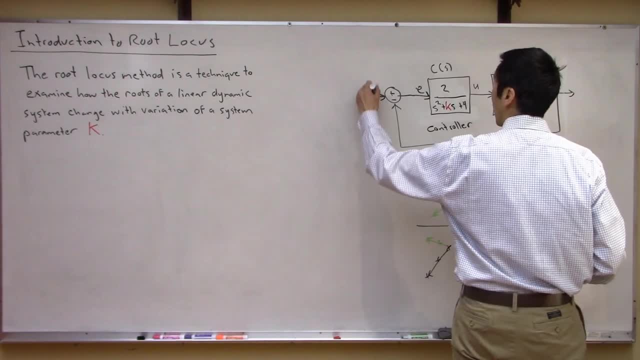 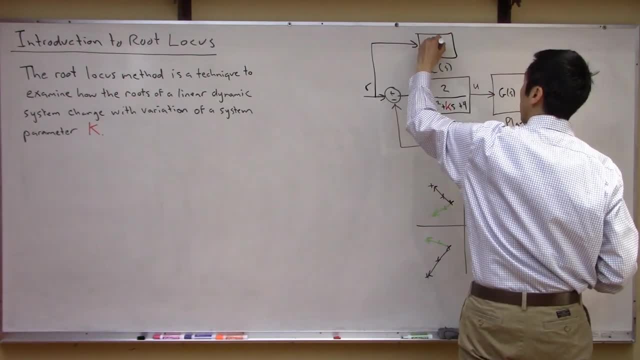 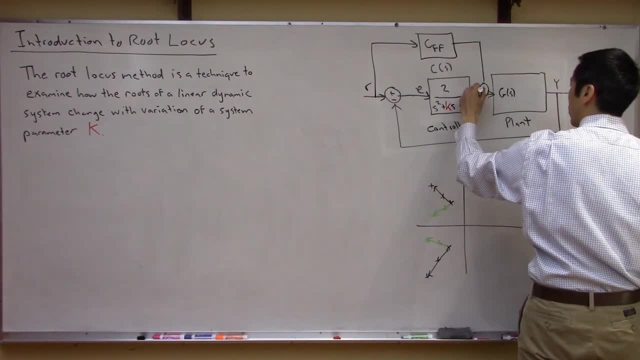 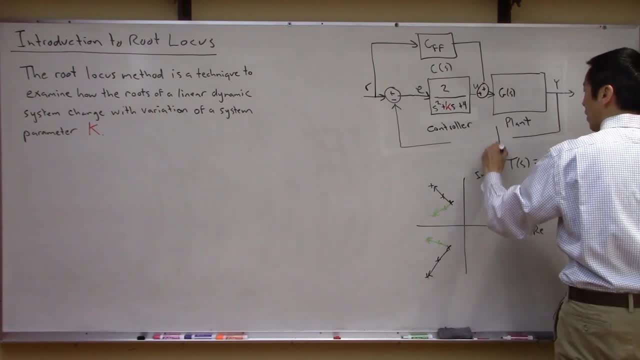 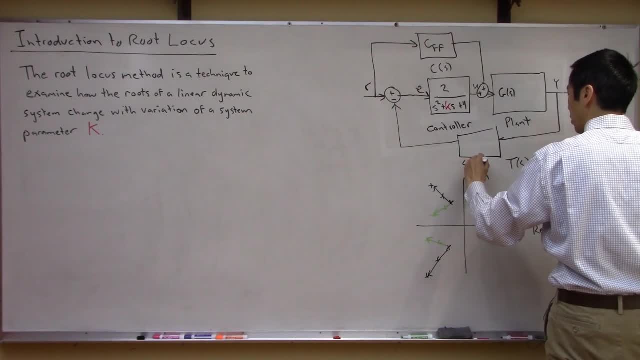 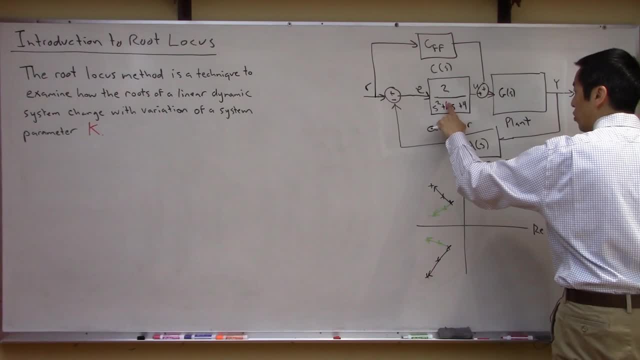 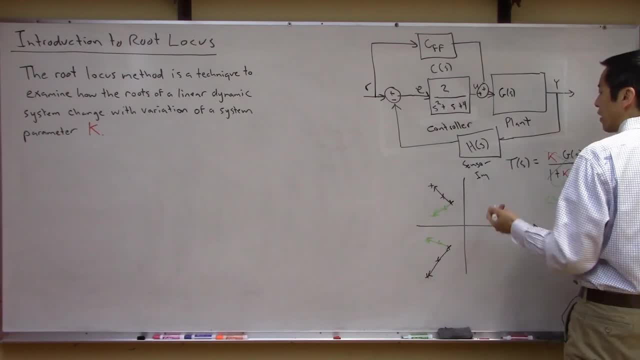 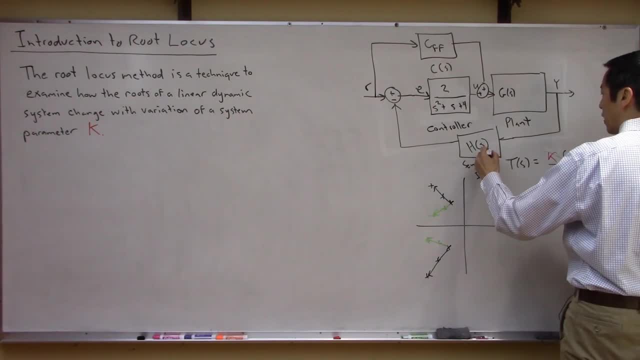 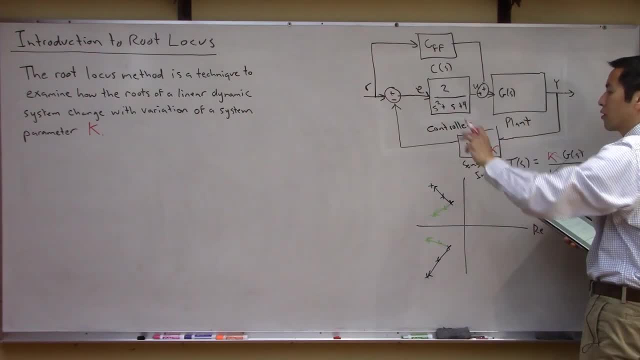 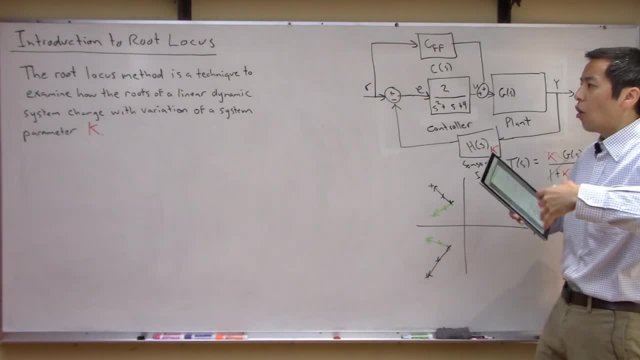 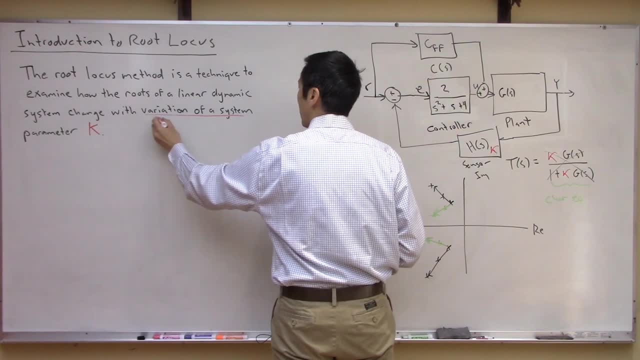 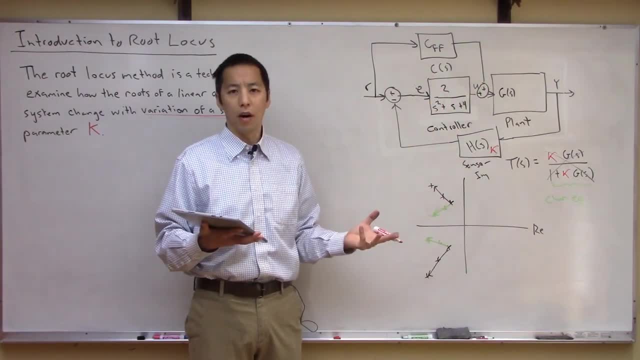 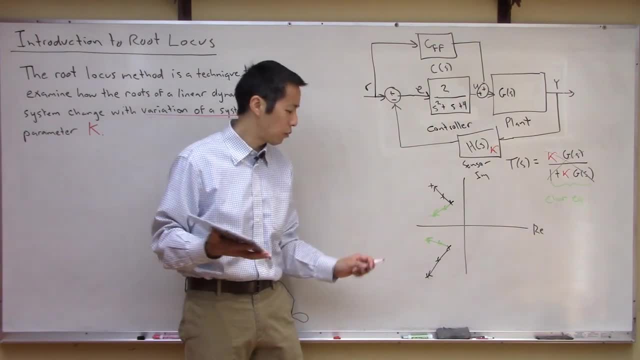 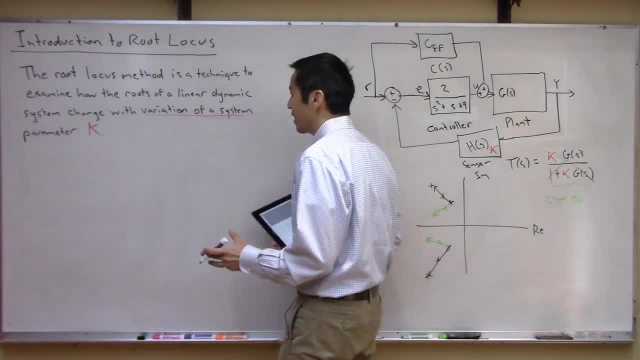 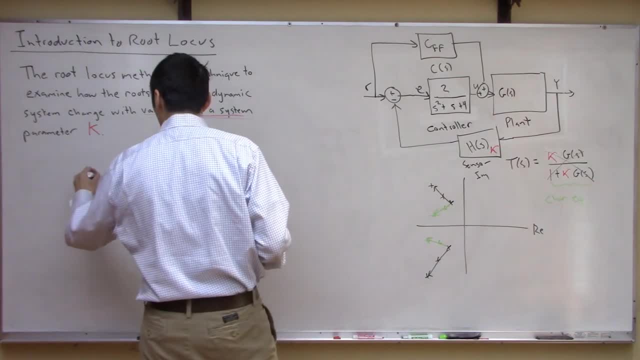 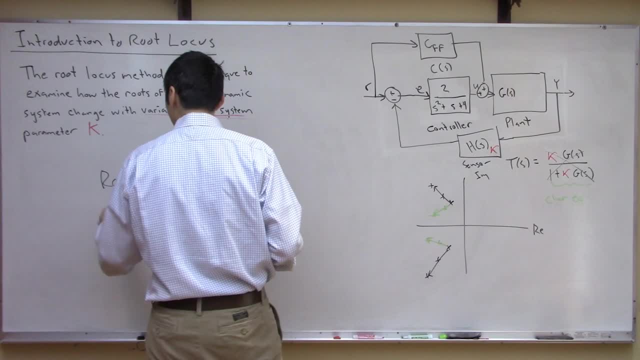 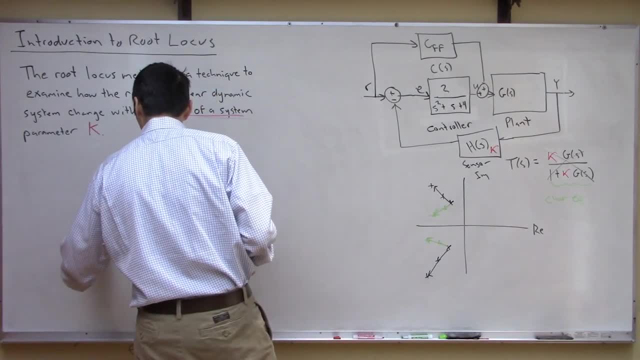 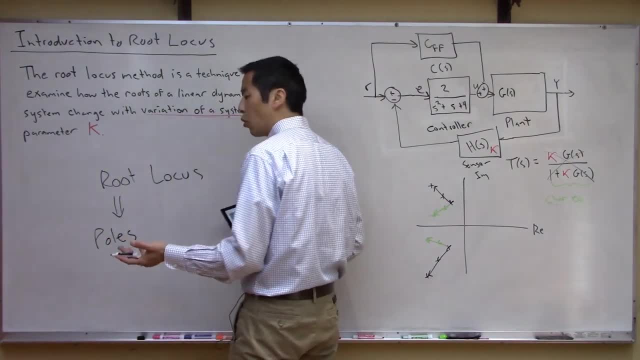 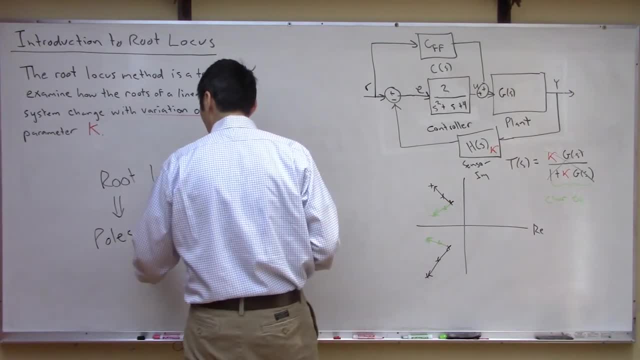 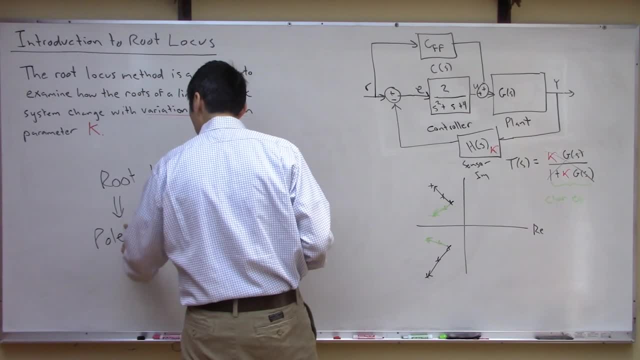 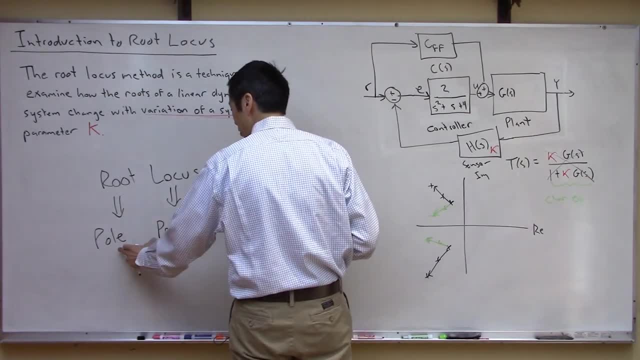 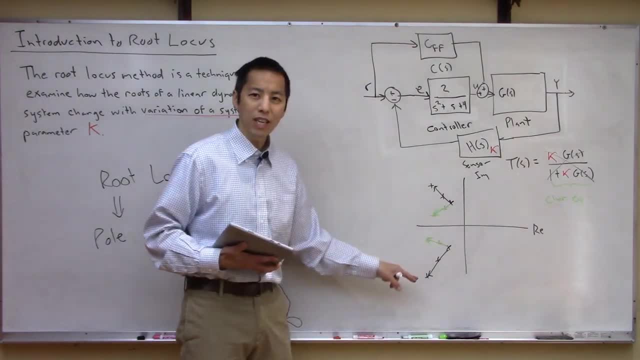 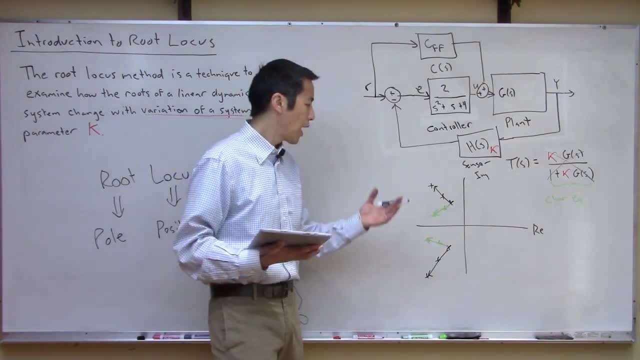 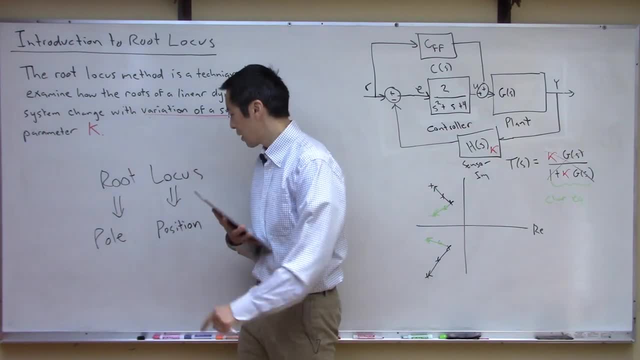 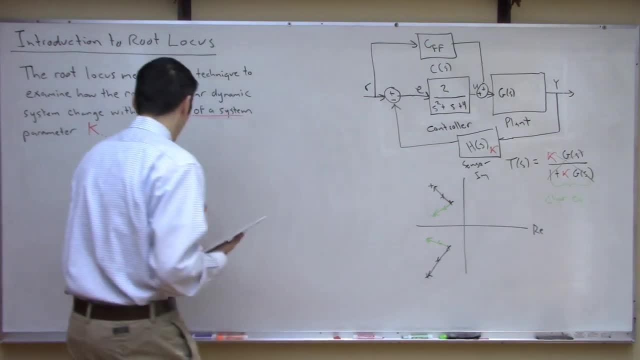 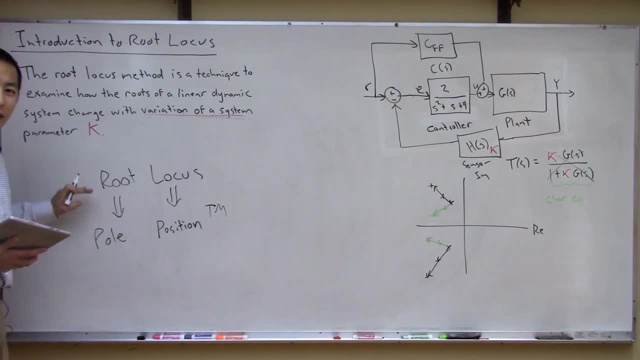 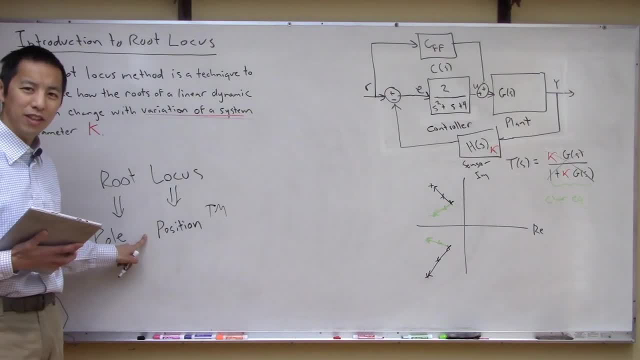 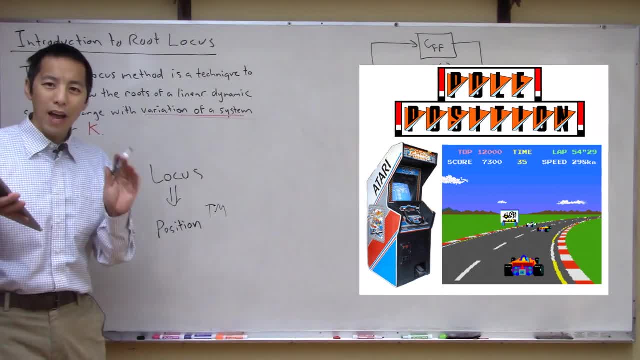 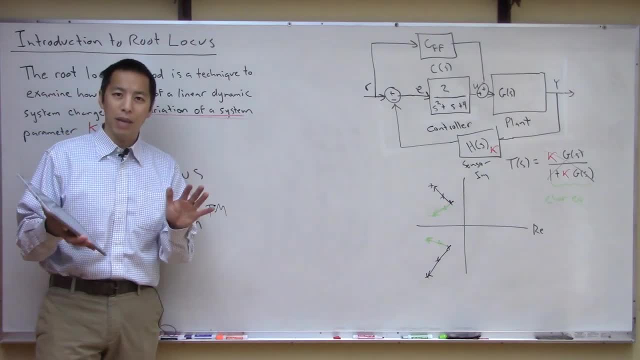 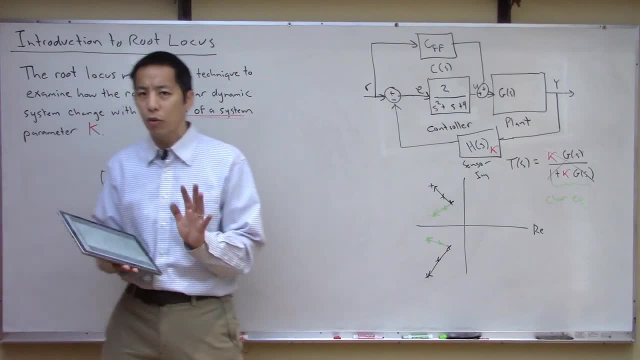 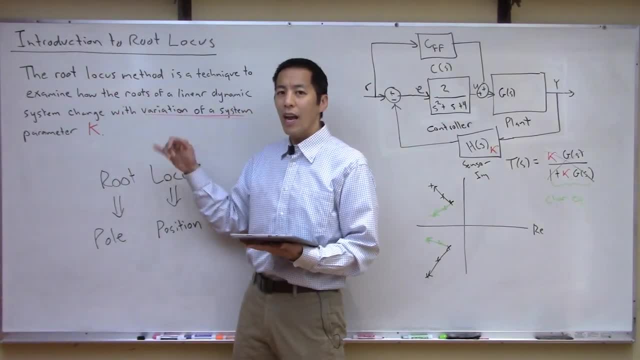 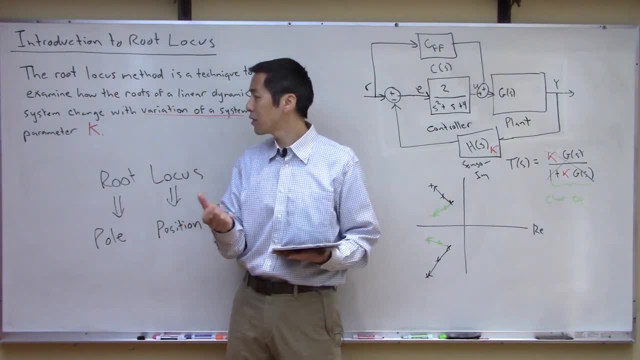 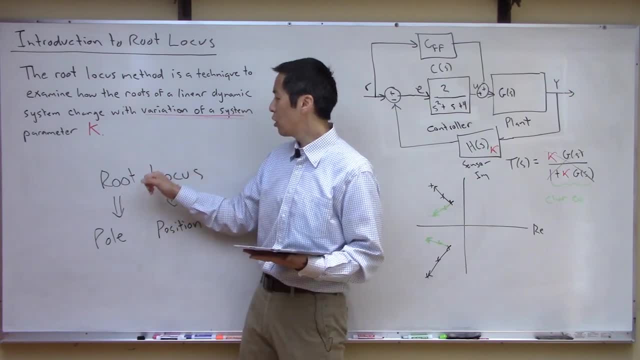 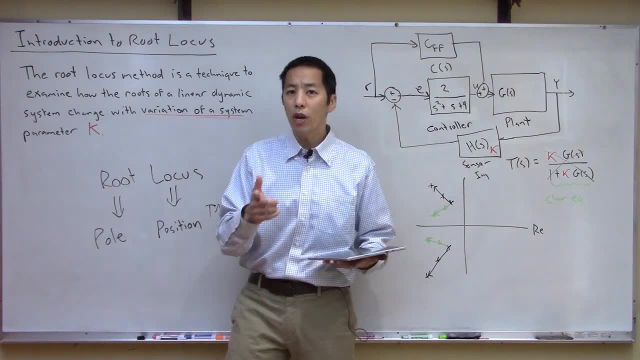 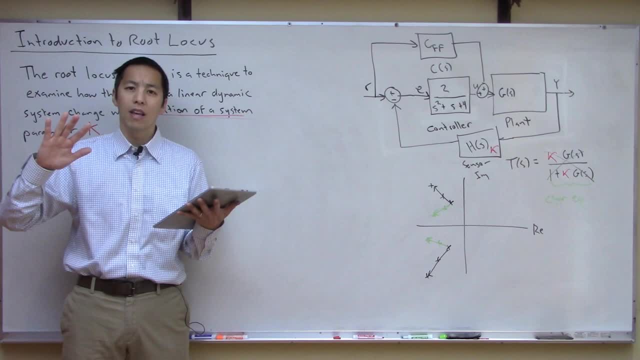 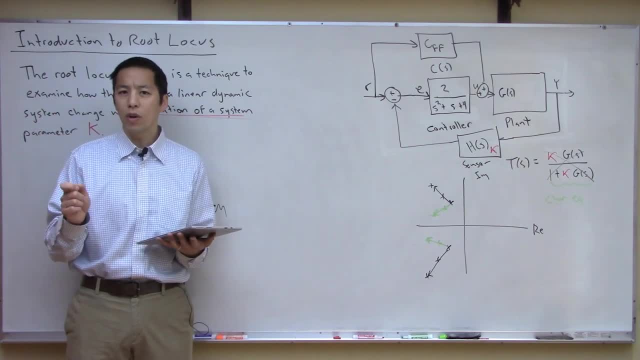 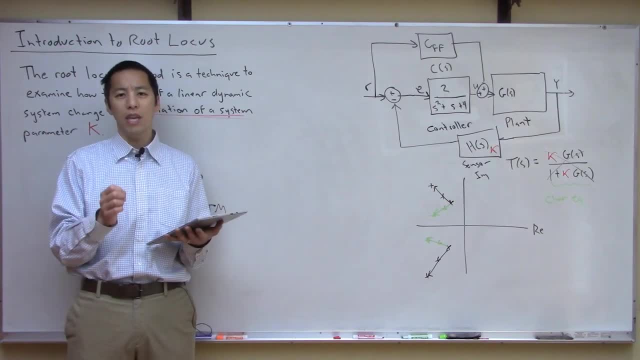 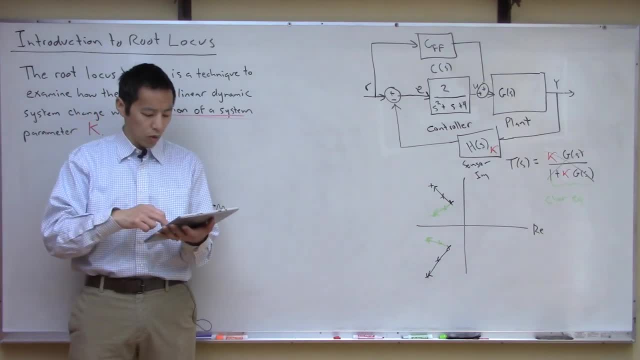 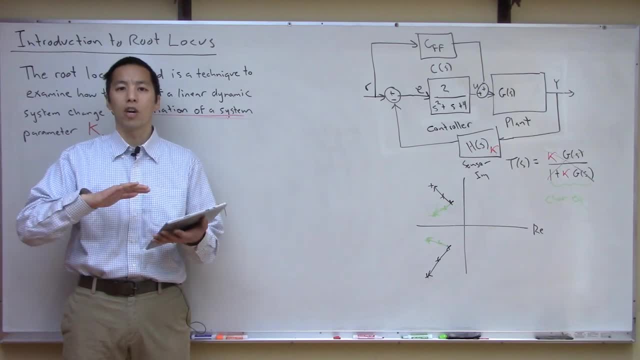 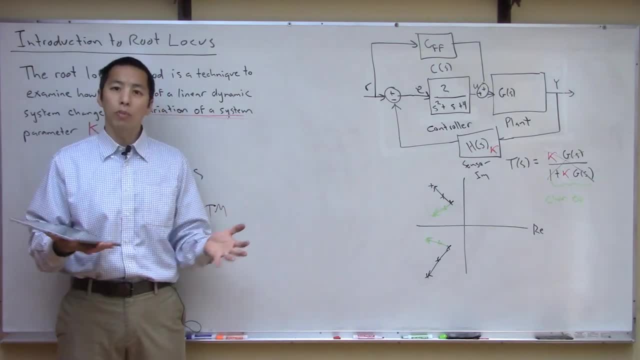 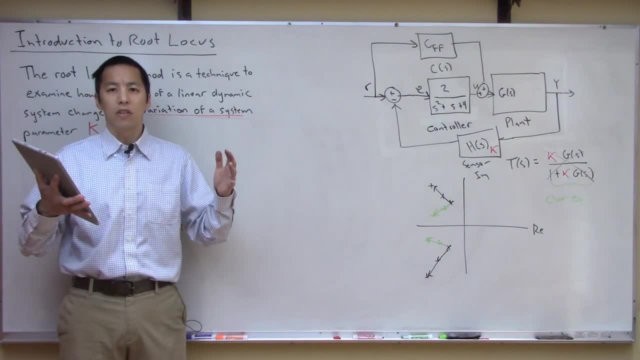 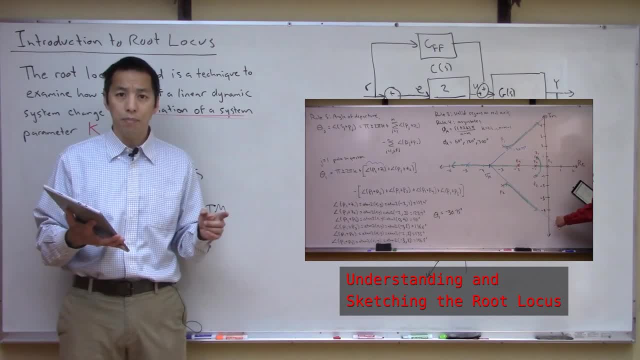 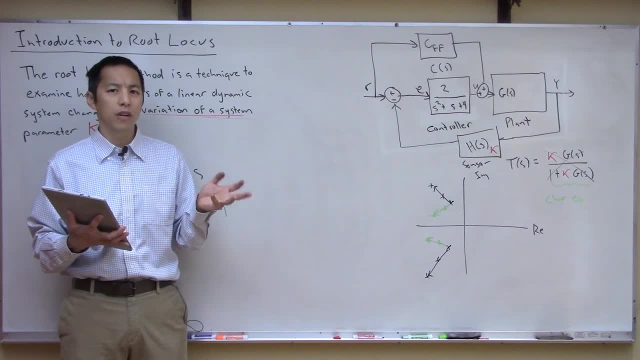 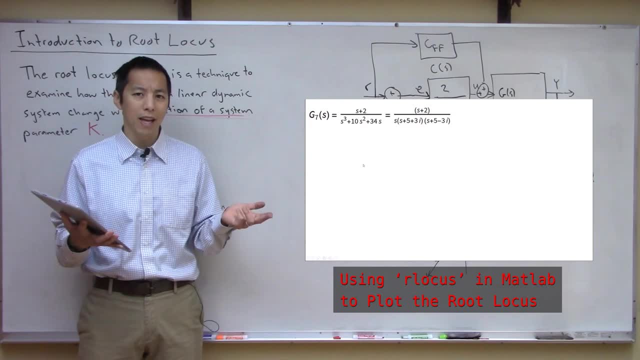 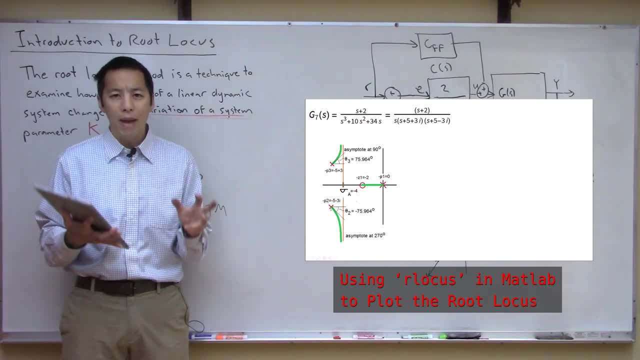 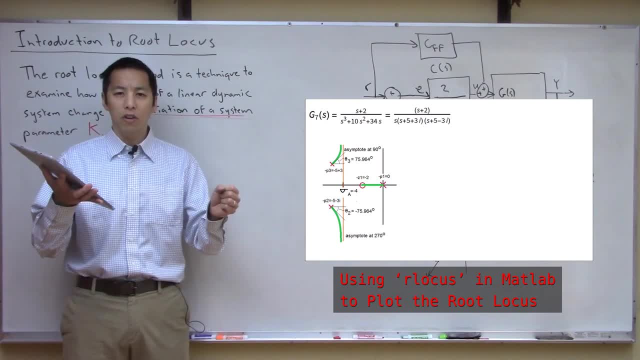 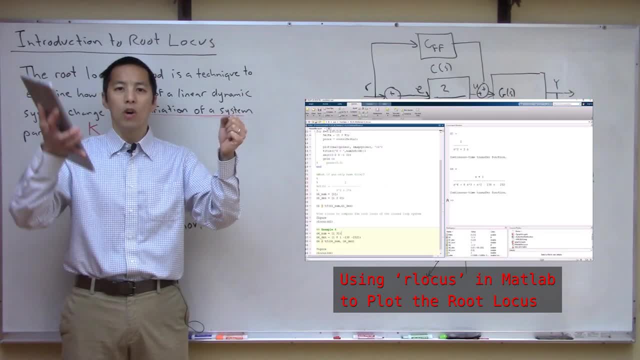 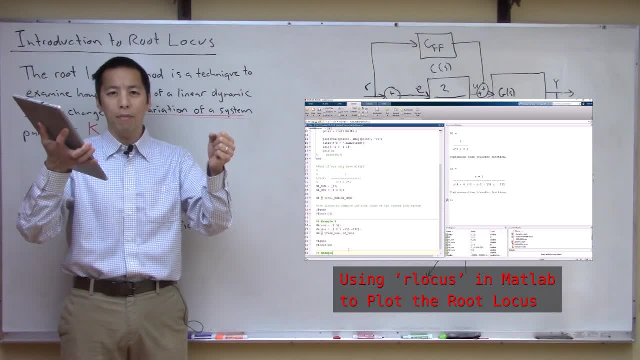 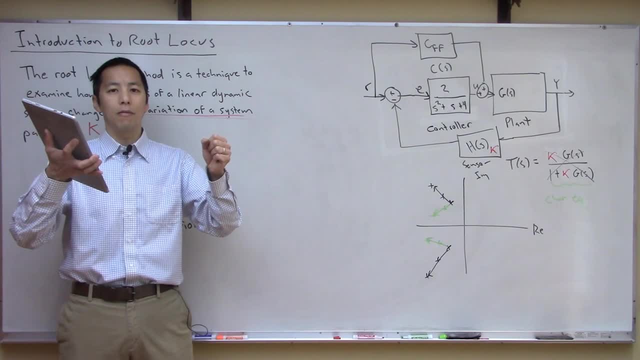 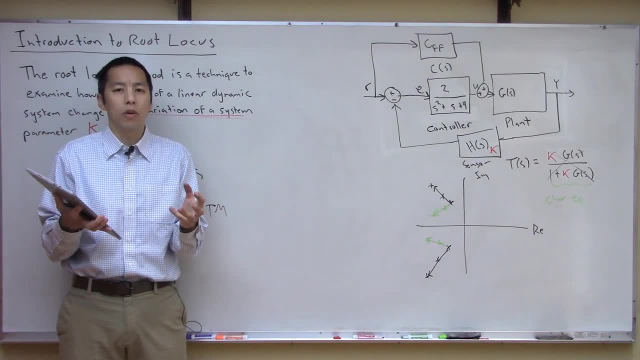 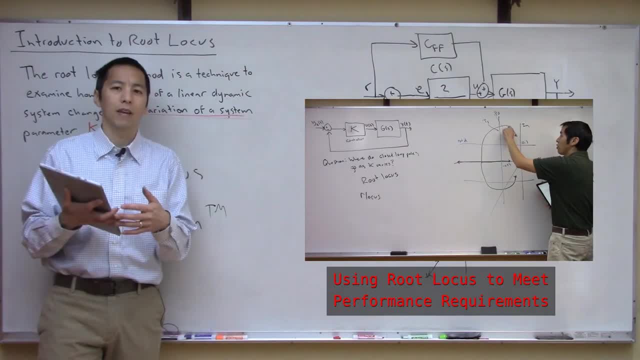 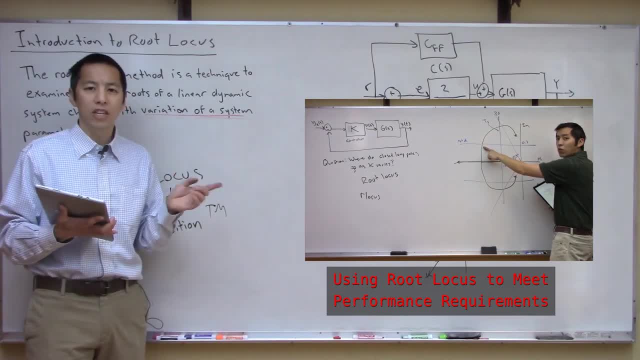 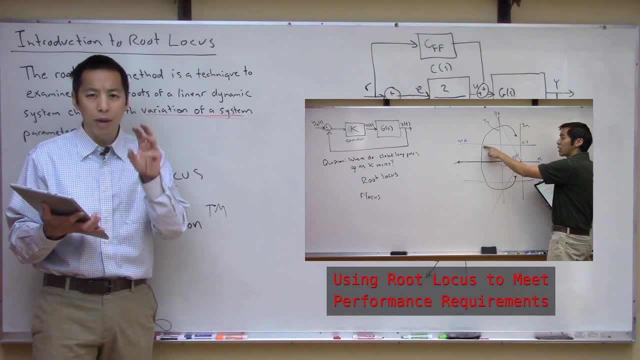 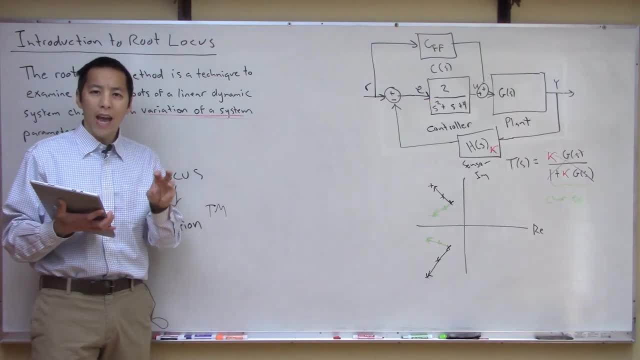 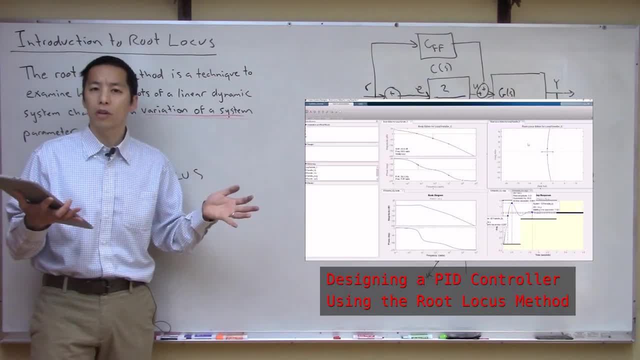 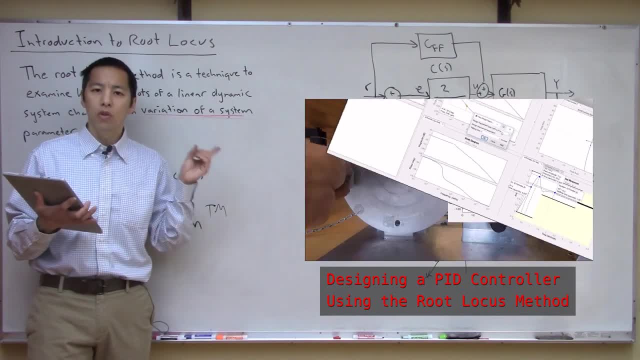 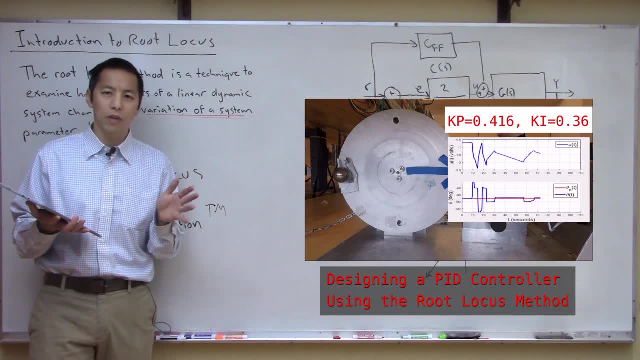 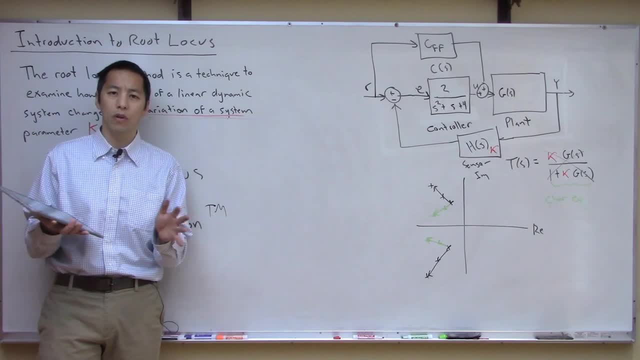 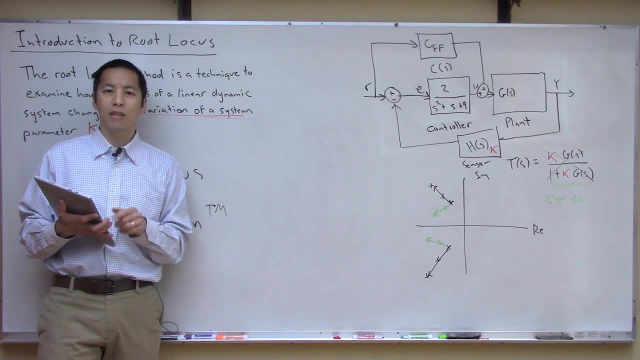